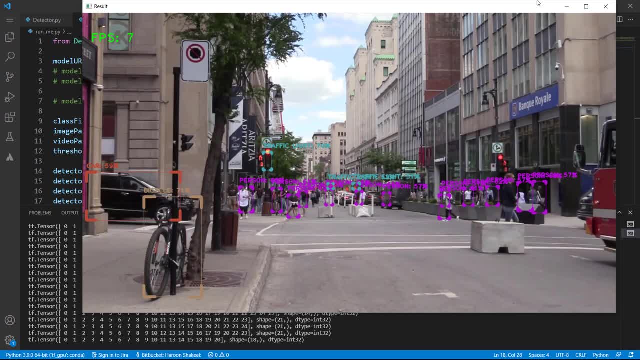 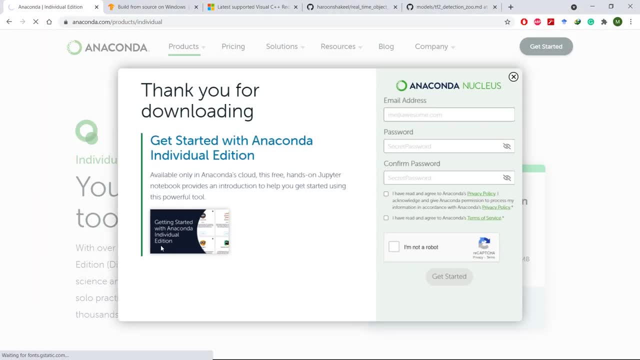 detector class for object detection on images, videos and webcam. You can find the timestamps in the description below. Let's get started. First thing that we need is Anaconda Python distribution. I am on Windows, so I am going to install using Windows installer, but if you are, 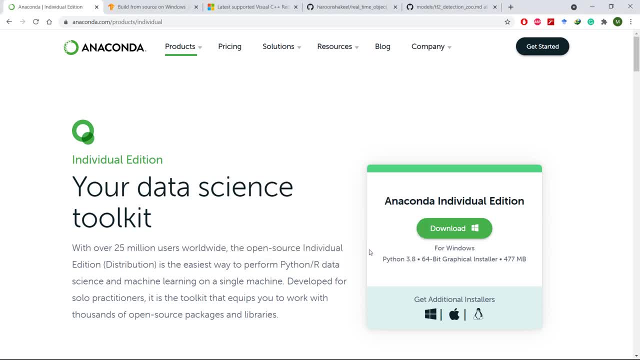 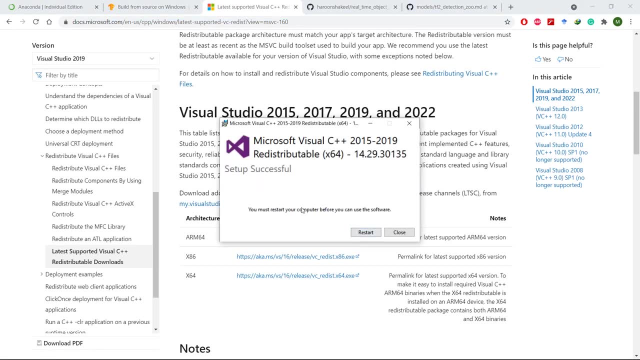 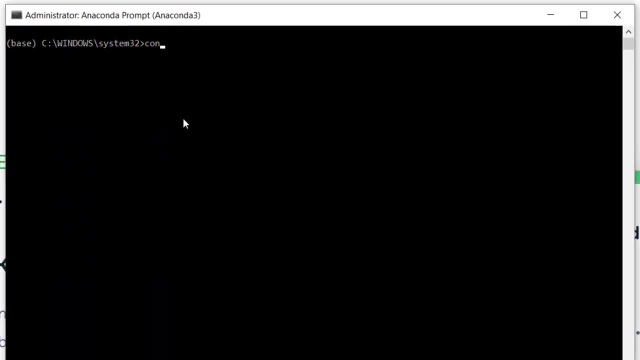 on Linux, use the respective distribution. Then on Windows, we need Visual C++ redistributables. Download and install Now open Anaconda prompt as administrator, because we will be installing a bunch of stuff Now. start by creating a virtual environment called tf underscore GPU. Let's create this. 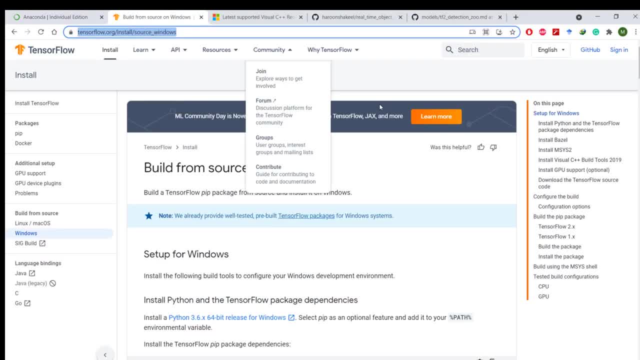 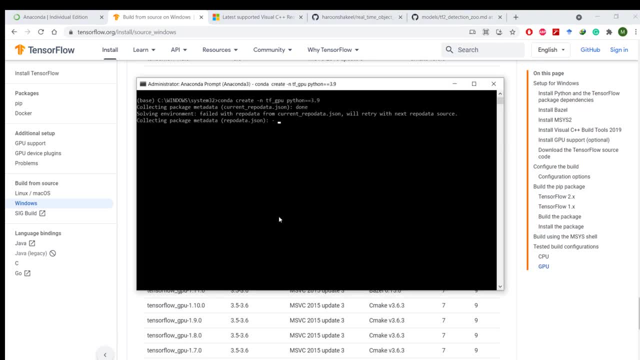 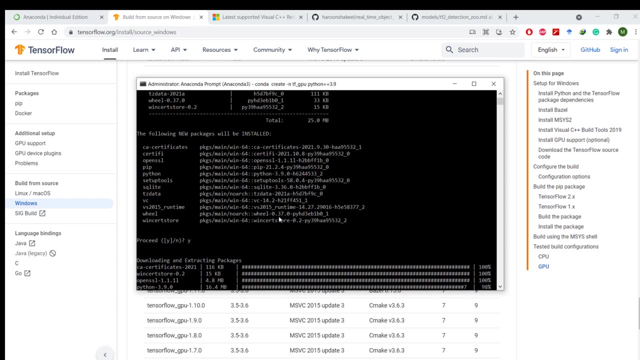 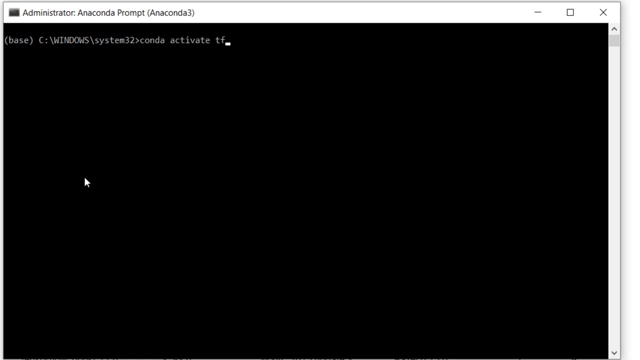 environment with Python version 3.9 because it is supported by the latest version of TensorFlow. Hit Y when prompted. Once Anaconda is done creating the virtual environment, Activate it by the command conda activate and then virtual environment name, which is tf underscore. 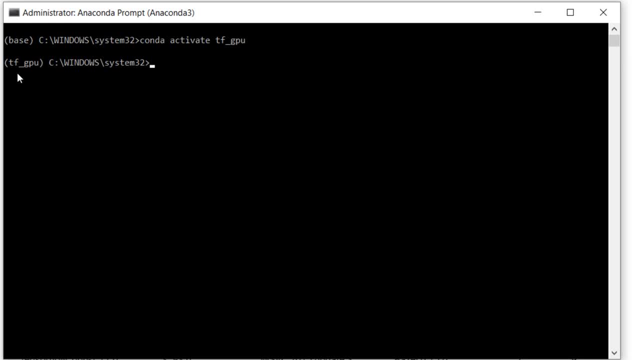 GPU. in our case Hit enter. Now we can see that the base environment is changed to our virtual environment. Let's clear the screen. So to install the latest version of TensorFlow CPU, first head over to the official tensorflow web page and install the latest version of Graham via persistence. 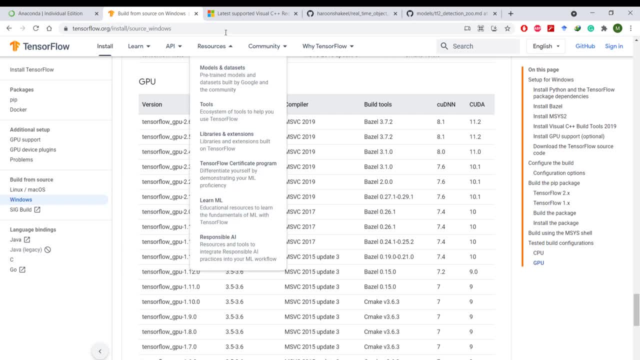 And if you close Doors then come into the wide嗯 WordPress virtual environment Can. and if we scroll down, we can see which version of CUDA and CUDNN are required for a specific version of TensorFlow. As we are interested in installing the latest version, we will need CUDA 11.2 and CUDNN 8.1. 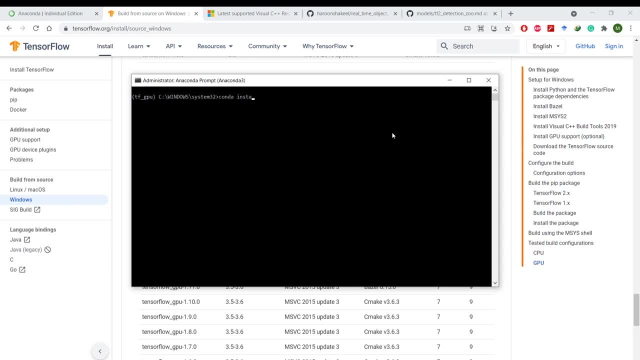 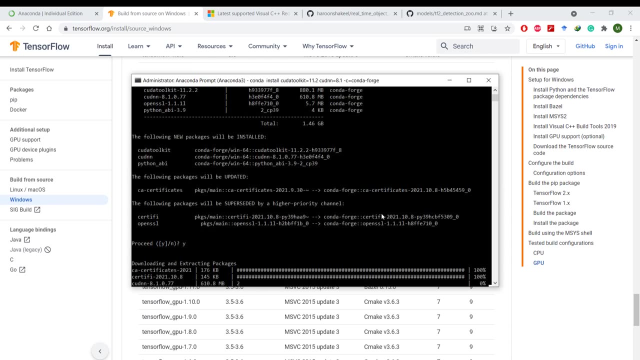 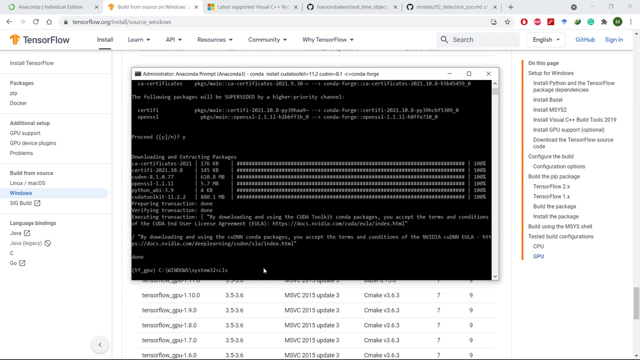 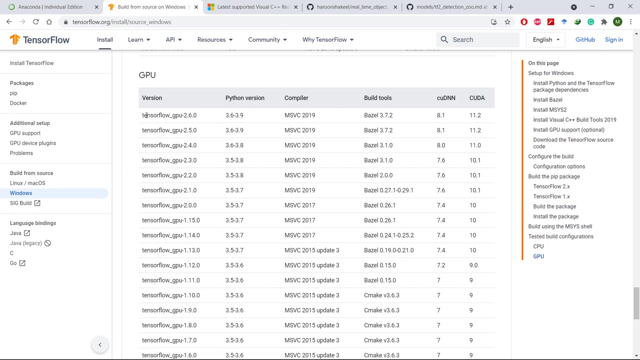 Let's install it by command: conda install CUDA toolkit equals 11.2 and CUDNN equals 8.1 minus C equals conda dash forge. Once that is done, now it is time to install TensorFlow. Let's install version 2.6, which is the latest version at the moment. so pip, install TensorFlow dash. 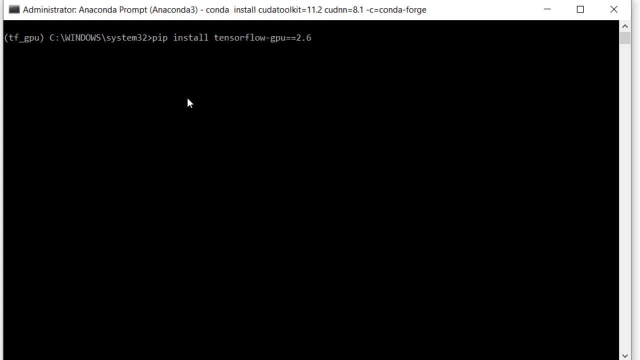 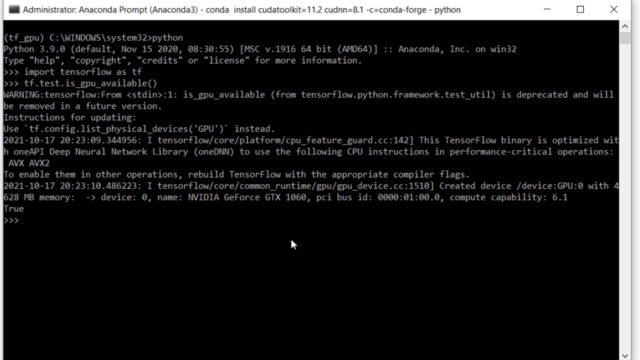 GPU equals equals 2.6.. It has finished the installation. Let's check if we have successfully installed it and our GPU is detected: run Python, import tensorflow and Then tftestis underscore- GPU underscore available. Everything looks great, but it says that this method will be replaced in the future, So let's use the other method as well. 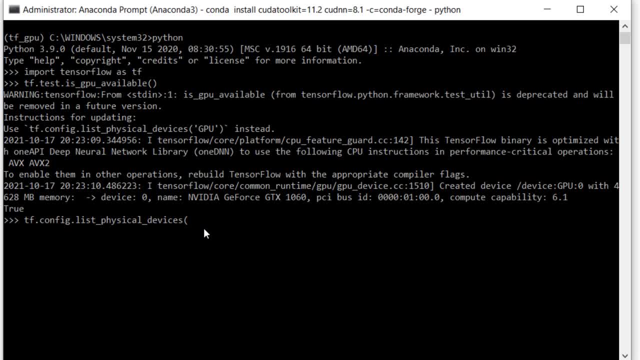 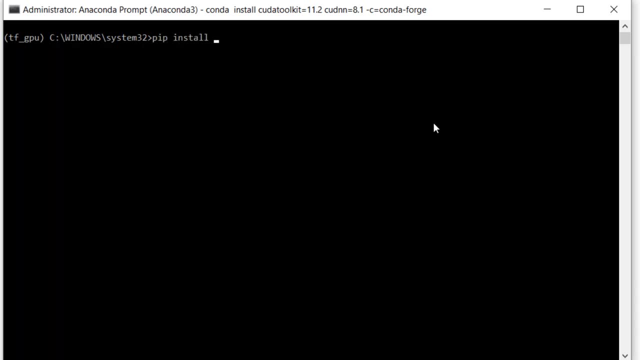 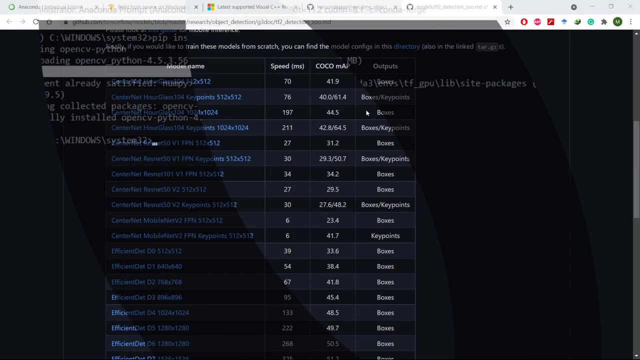 So It also detects the GPU. Finally, we also need to install opencv for loading the images and videos. Let's install it by command: pip install opencv dash python. That's it. Our development environment is all set Alright. we will be running all these models that are available at tensorflow. 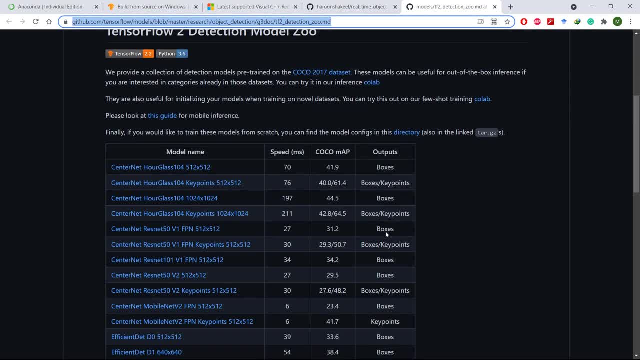 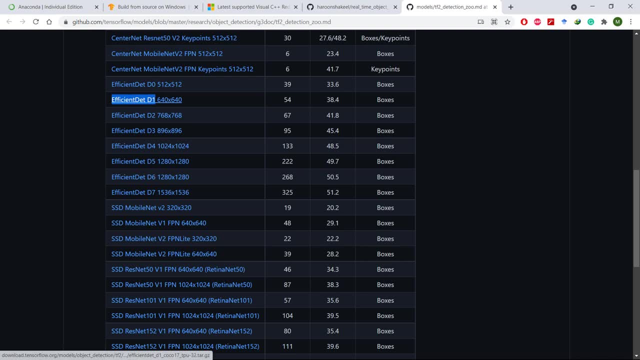 object detection Zoo. these include all versions of efficient debt, SSD, mobile net and faster our CNN. these models are trained on coco object detection data set and There is always a trade-off while selecting a particular model. For example, there are some models that have lower inference time, so are suitable for running on CPUs or mobile devices. 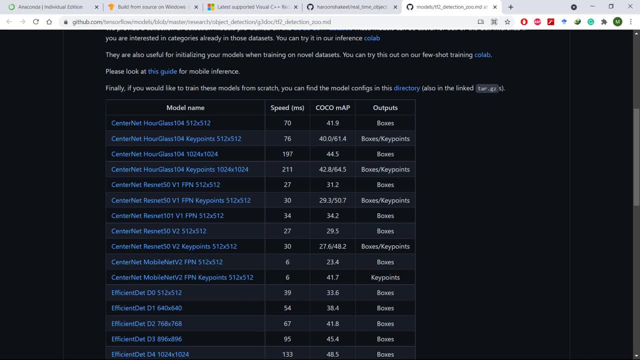 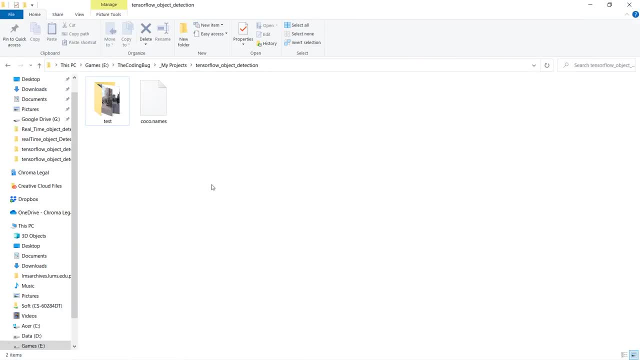 But they have a lower performance. Some have higher inference time but are also more Accurate. so the choice of the model really depends on our use case. Okay, so let me show you what I have got here. I have a test folder with a bunch of images and videos that we will be using to run the object detection and 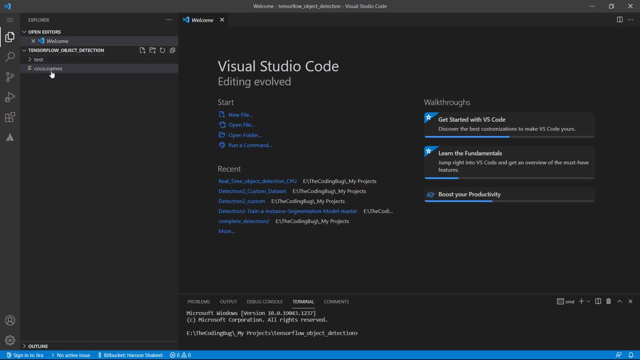 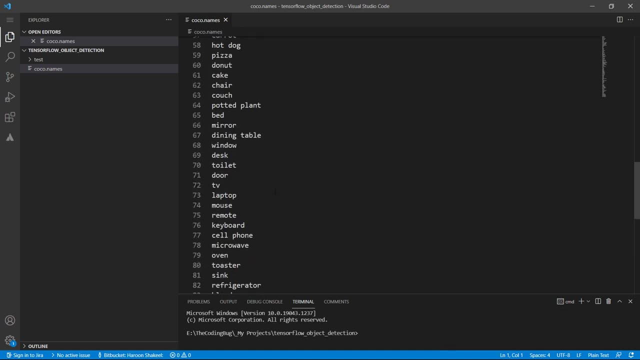 There is a file called coco dot names which is available officially with coco data set. I will put the link in the description. This file contains the names of all the classes on which all of the object detection models are trained. There is one edit that we are going to do. first class label for this file should be background. 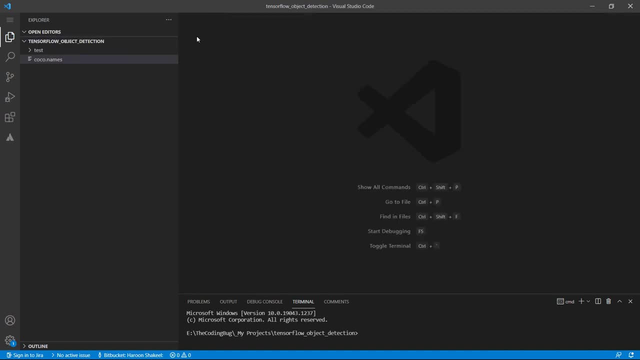 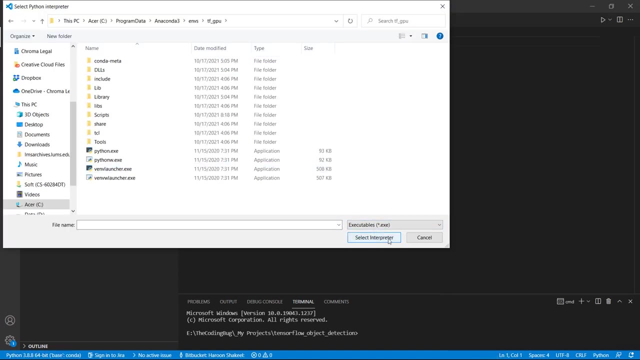 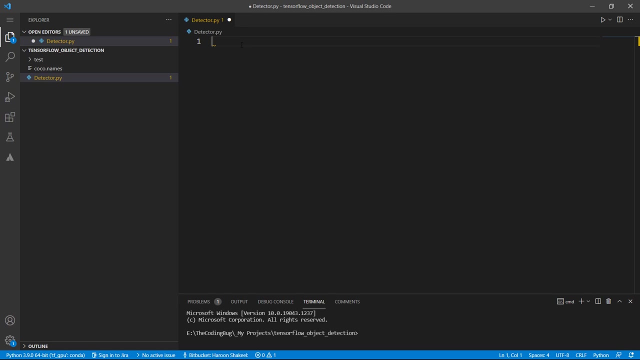 So let's add it and save the file. Now let's create an empty Python file called detector dot pi. Vs code is asking to select Python environment, So let's select TF underscore GPU environment that we have created in our detector dot pi file. import CV to time OS and. 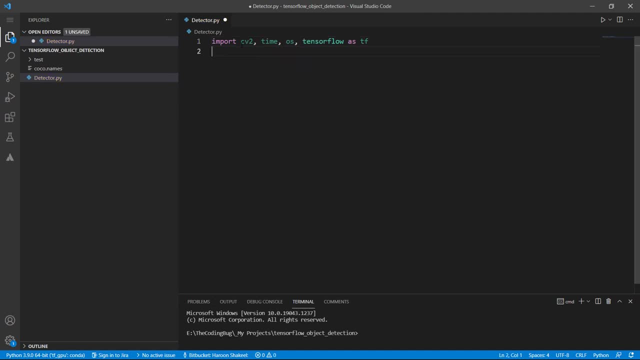 tensorflow as DF. also import numpy as NP and from tensorflow dot, Python, dot, keras, dot utils, dot data underscore utils, import, get file. Let's fix the random seed of numpy to, let's say 1, 2, 3, so that we get reproducible results for all the runs. 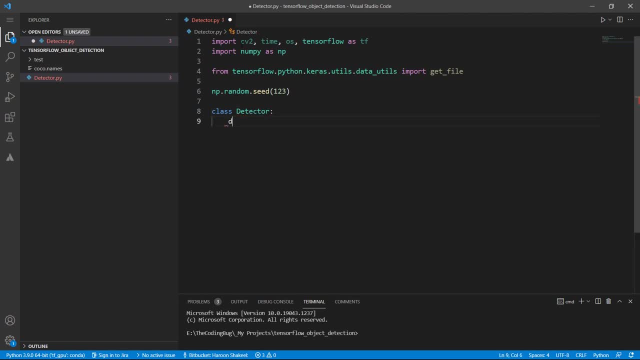 Now we will start implementing the detector class. Let's define init method, Which will be empty, so just pass it, as we are not implementing anything in this method. Now we need to read the class names file. for that, Let's define read classes method, Which takes class file path as argument. 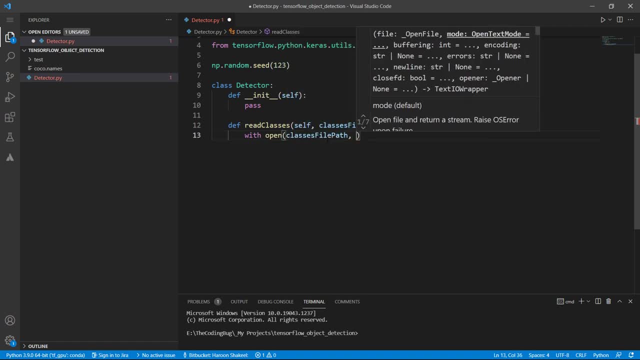 We will be opening this file in read mode and then split all the lines and put the text in a list. We are calling this list self dot class list. so remember: any variable with Prefix self is available anywhere within the class. Now we also need a unique color for every class label. 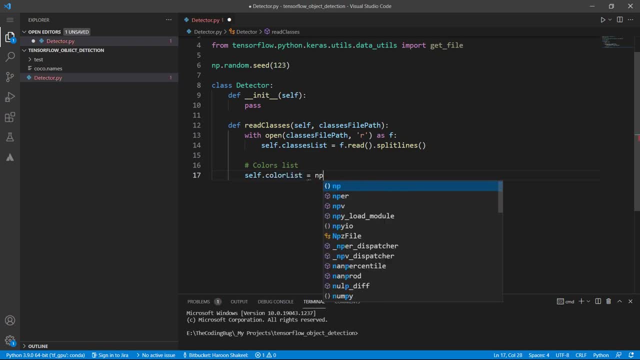 So we can randomly initialize color values using NP, dot, random dot, uniform. give lowest value 0 and highest value 255, and the size of this list would be equal to the length of our class list and There would be three channels. great, now let's print the lengths of class list and. 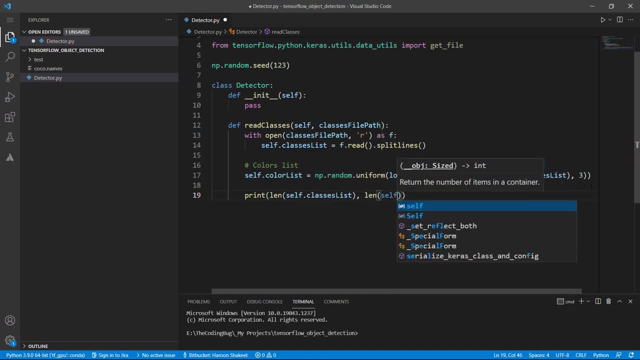 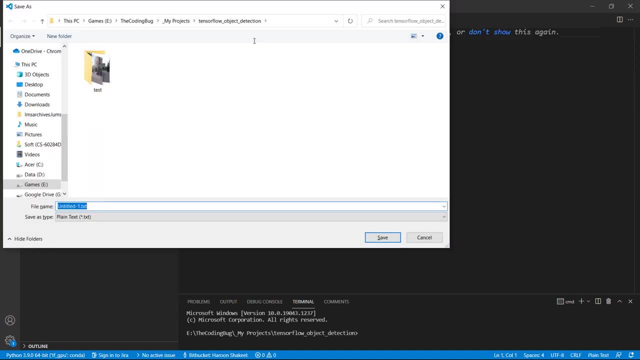 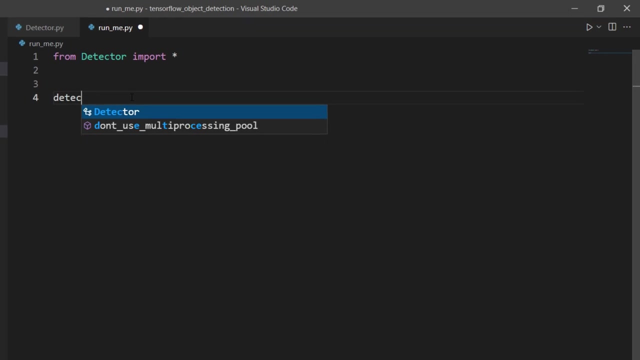 Color list to see if both are equal. Okay, now we need the driver program. so let's create another empty Python file called run underscore me dot, pi and import everything from detector class. let's initialize detector class and create an object called detector and Call this read classes method. It takes classes file path as parameters, So let's define that. 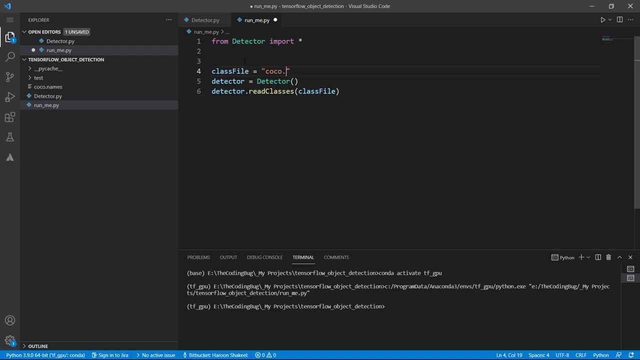 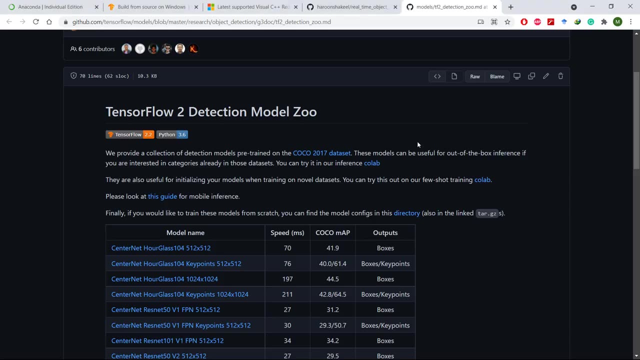 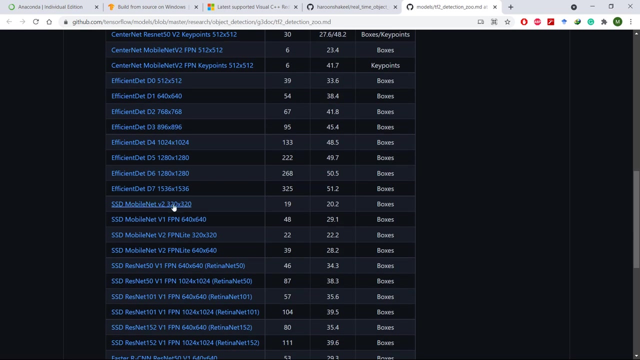 class files equals Coco dot names. Let's run the code and here we have 92 classes and 92 colors. Now we have to download any model from the model zoo. So suppose we want to run SSD mobile net v2. So just copy its link and let's save it in a variable called model URL. 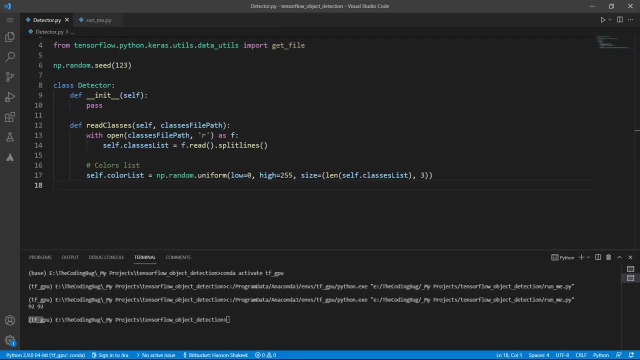 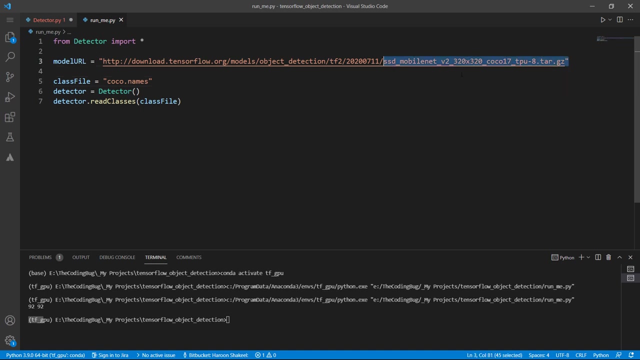 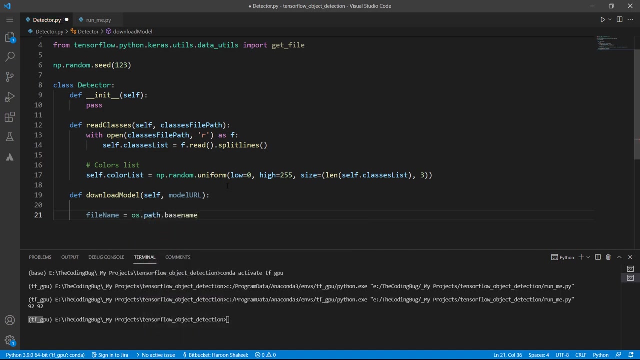 Now head back to detector dot pi and define a function called download Model, which takes model URL as an argument. We already have model URL, but we need to extract file name from it. It's this last part with dot, tar, dot gz extension. We can get that by using OS dot path, dot base name and it will give us the file name. 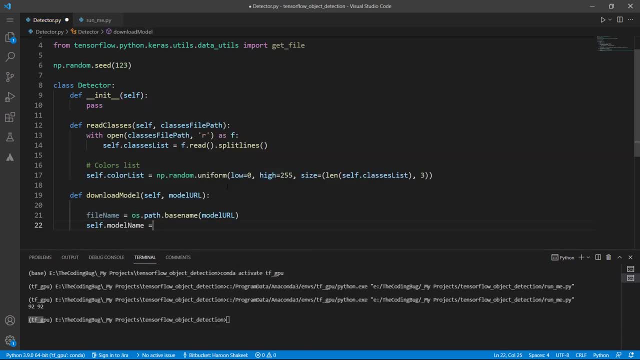 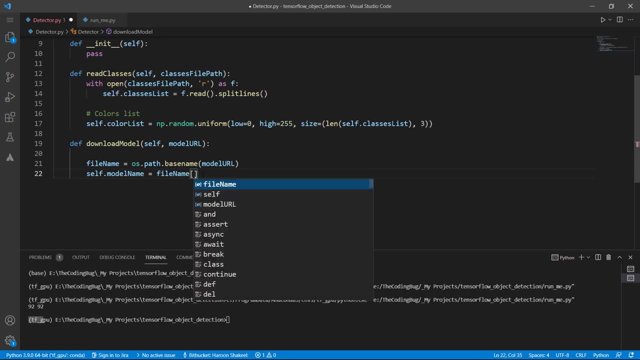 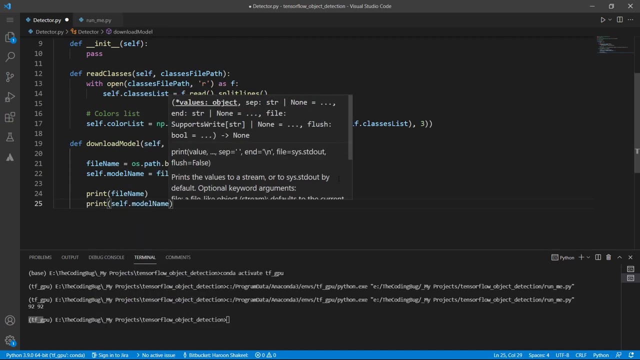 From this file name. We also want to extract the model name, which is this part without the extensions. We can do that by taking the characters of file name till we hit the first dot. Let's print the file name and the model name and see what we did. 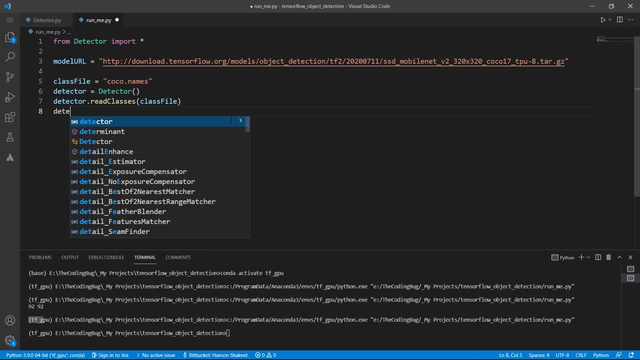 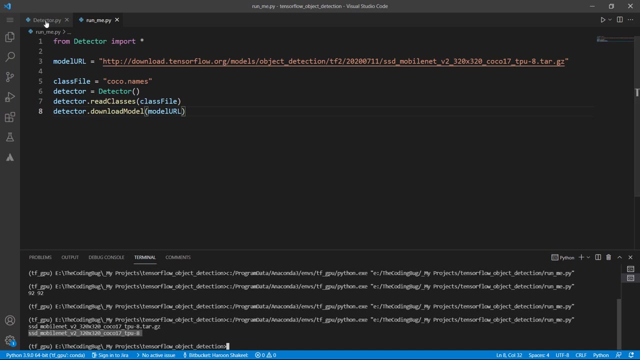 In main file. let's call download model method and pass the model URL and run the code. Here we can see that we have extracted the file name and model name successfully. we will be using this information in subsequent code. now we define a cache, a directory where all the models will be downloaded and stored. so I am defining 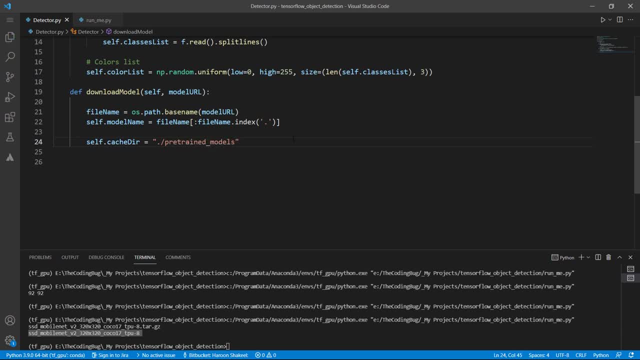 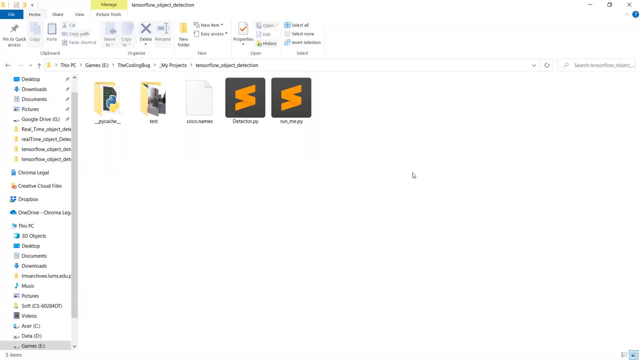 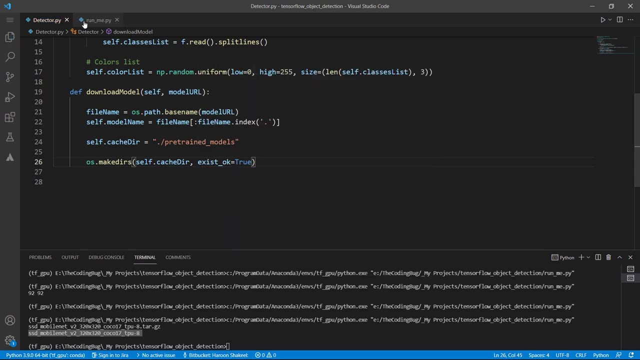 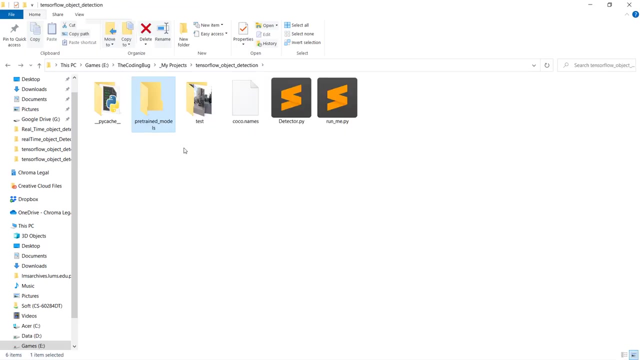 dot slash pre trained underscore models, which means that the cache, a directory, would be created at the same place where we have placed the detector dot PI file. we need to create this directory and if it already exists, we will skip it. let's now run the main file and we can see that this directory is created. now we 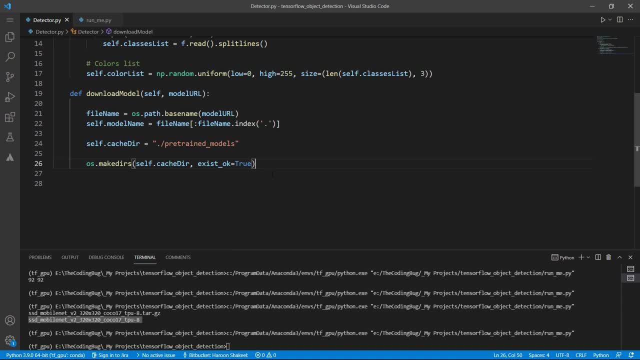 will use get file method to download the object detection model. so let's call get file and then pass the file name that we just extracted above. after that we have to pass origin URL, which is stored in model URL parameter. then we need to tell here is the directory that we have created, and then we need to pass the. 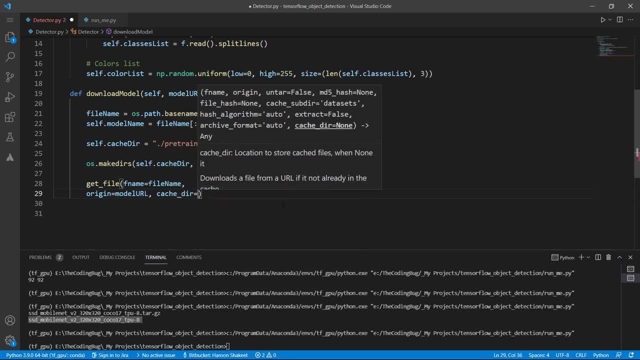 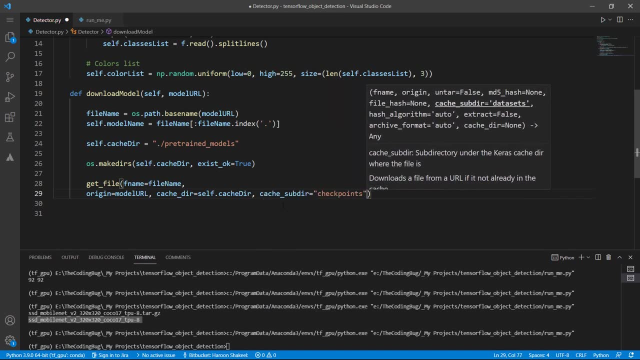 cache a dir where the model will be downloaded, it's self dot cache a dir and then sub directory inside cache a dir, which I am defining to be checkpoints, as the model will be downloaded as an archive. we want to extract that, so now let's run the main file. we can see that SSD mobile net is being downloaded from. 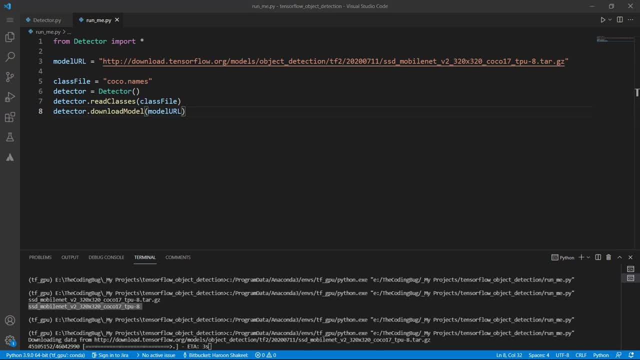 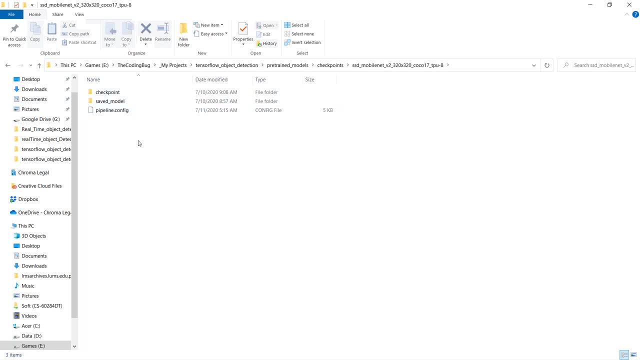 tensorflow object detection model zoo, because that is not present in our cache a dir. in the cache a directory we can see that the object detection model is not present. in our cache a dir we can see that there is a checkpoint directory and the model file is downloaded and extracted. if we run the code again, this: 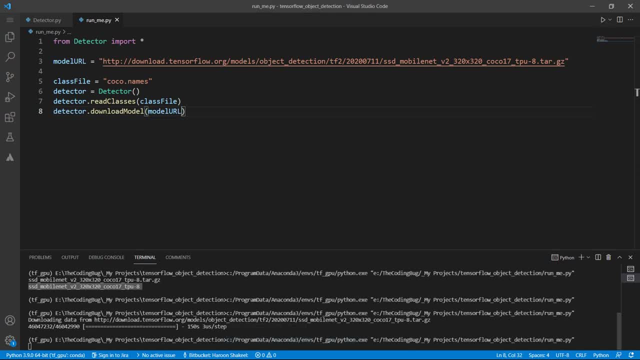 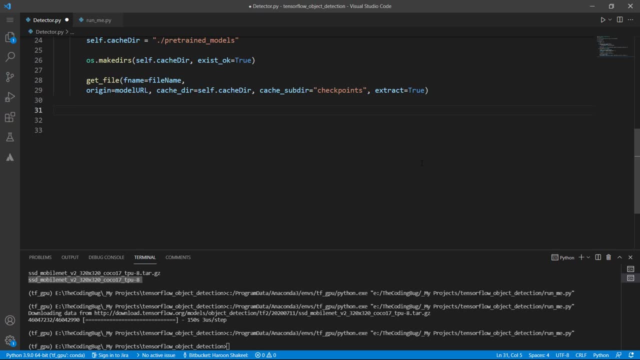 time, the model will not be downloaded as it is already there in our cache. a once the model is downloaded, we need to load this model using tensorflow. so let's define another method called load model, and here I am printing the message loading model and then concat the model name. okay, now let's go to the next step. 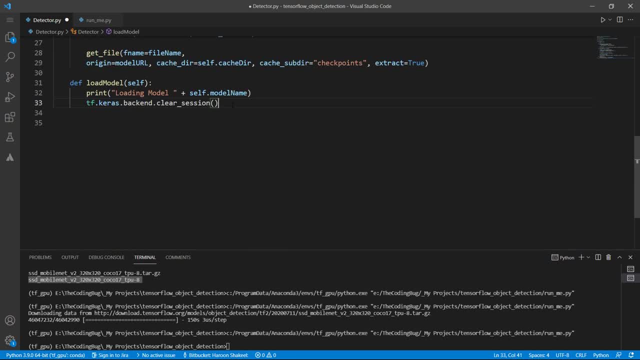 let's clear the keras session and load the model in a variable called self dot model. let's call tf dot saved underscore model dot load. we need to give complete path to the extracted object detection model, so let's use os dot path dot join. then there is cache a directory, then checkpoints folder and model name. 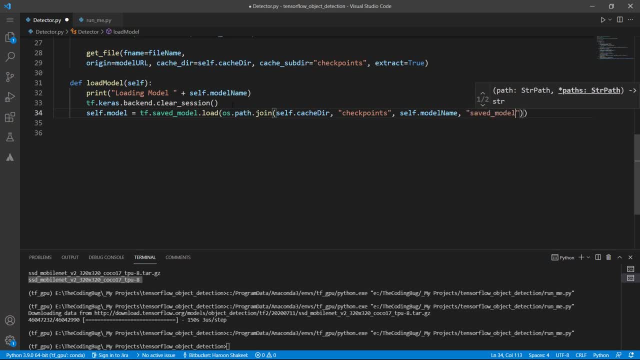 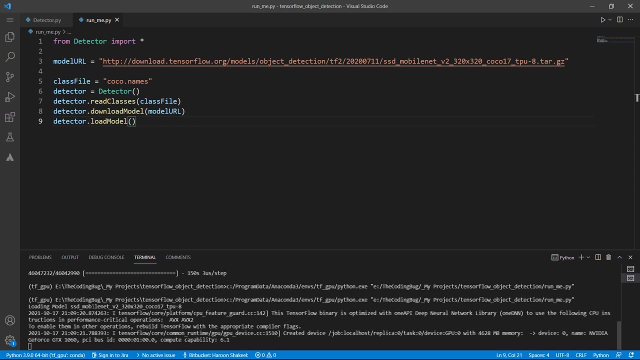 and finally, we have saved underscore model folder. so basically I am mentioning the directories that contain the saved model. let's print the message that model is loaded successfully. let's call load model method in main file, and here we can see that the model is loaded successfully. so it's working great. so. 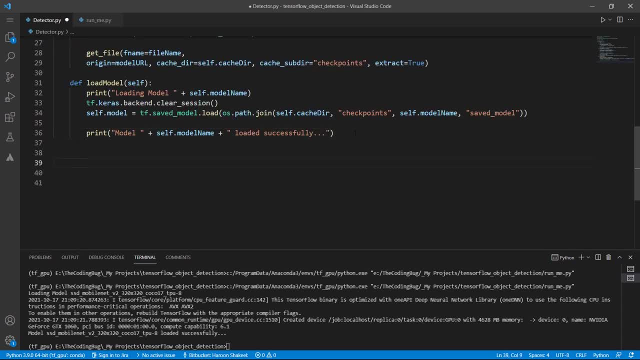 far. now it's time to make some predictions on the image. so let's define method called predict image, which is the image that we are going to be using for the project. so let's say we are going to create an image which takes image path as input, read the image and place it in a variable called image. let's show the. 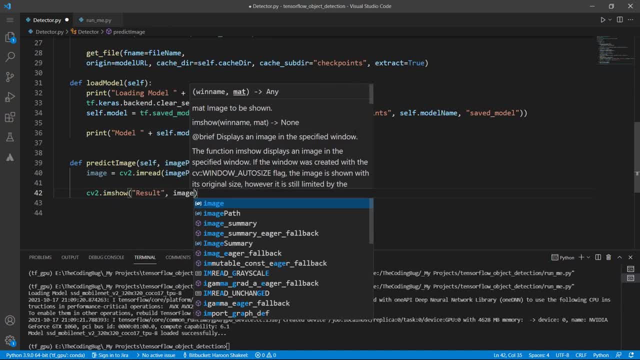 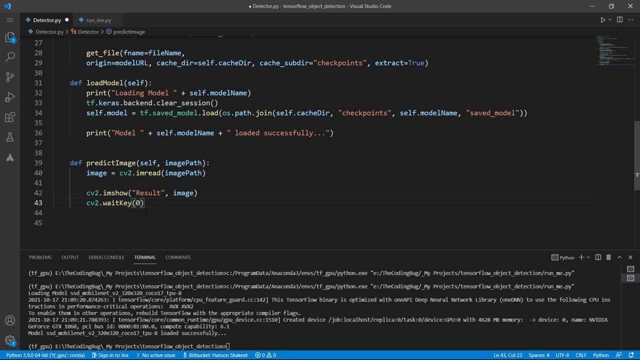 image using cv2 dot, I am sure- and then wait for a key press. so 0 here means that we will be waiting indefinitely. but if we pass any integer, let's say 10, it means that cv2 will wait for 10 nanoseconds for a key press. and finally, 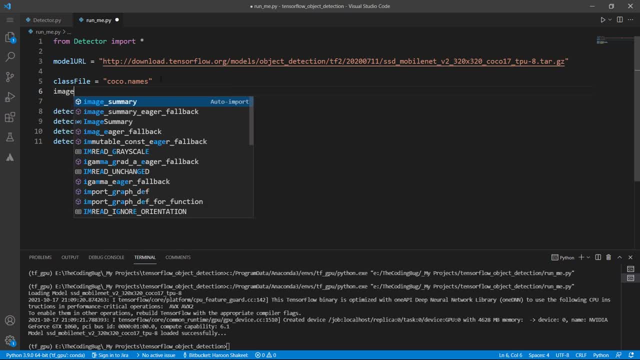 destroy all opencv windows, let's say 10, and then we are going to create a new image. so let's define image path in the main file and call predict image method and pass the image path as parameter. here we have the image. of course we have not. 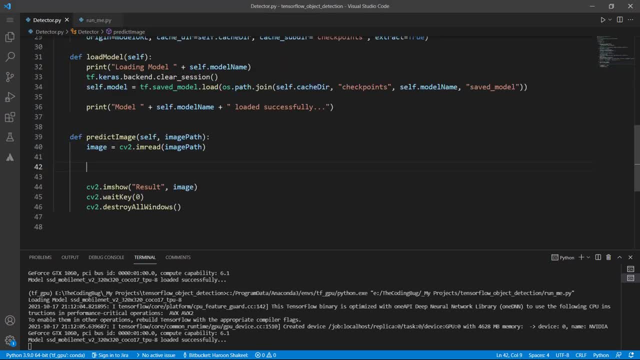 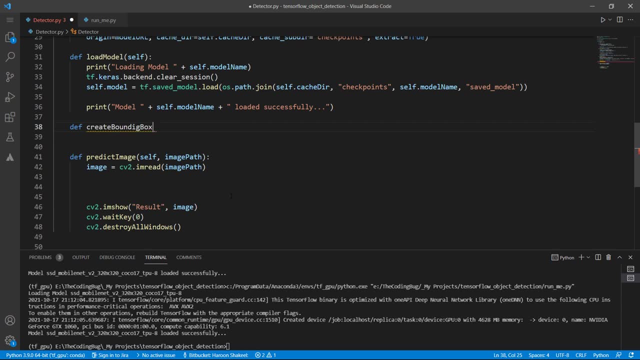 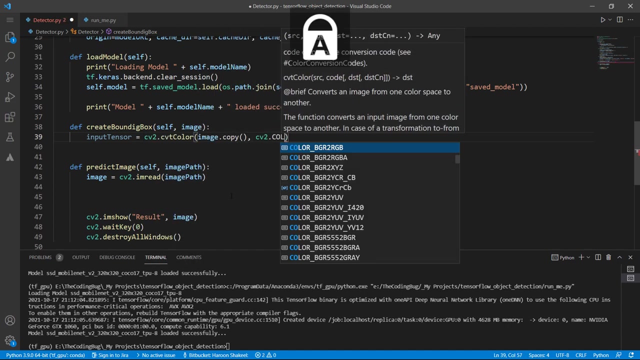 performed any object detection yet. so no bounding box is there. let's define another method above which takes the image as input and makes predictions. we are gonna call it create bounding box, and it takes image as parameter. this image is loaded by opencv in BGR format, so let's convert it to RGB format and 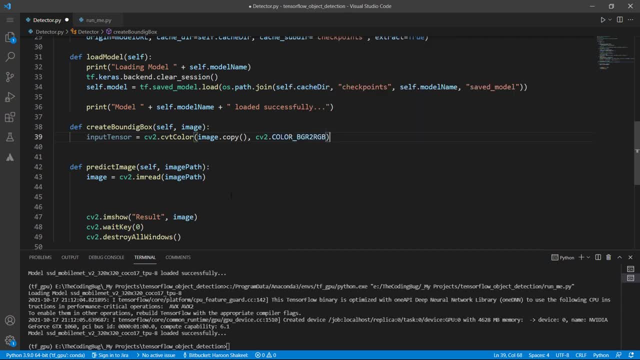 call it input tensor. this is a numpy array but we need to convert it to tensor and tf dot convert underscore to underscore tensor method will allow us to do that and its data type would be unsigned, integer 8. so tensorflow takes a batch as input. so this is just one of the parameters. we need to convert it to a. 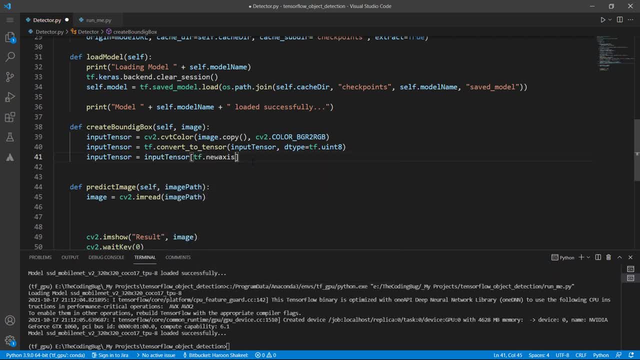 one image, so this should be batch of one. so we need to expand its dimensions. there we go. now we pass this input tensor to the model and get detections. these detections are a dictionary, so we need to extract bounding boxes and convert it to numpy array, extract class predictions, which are basically index of 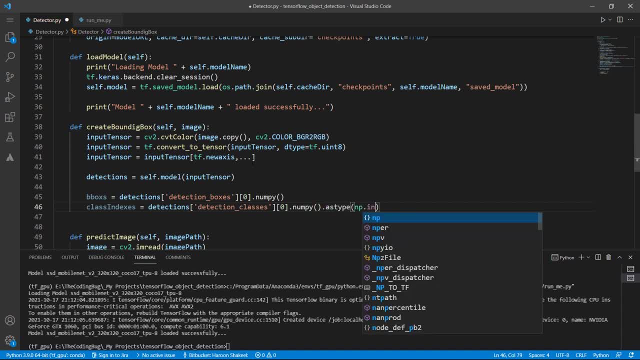 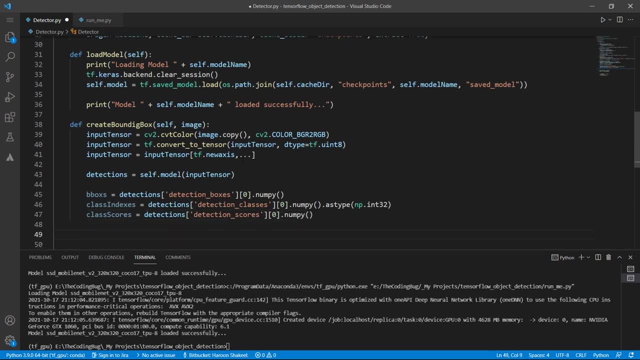 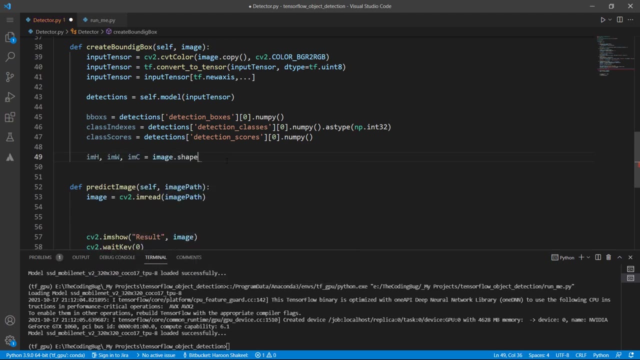 the class labels and let's convert it to integer array, then extract the confidence for each class label and convert them to numpy array. now let's determine the image height, width and the number of channels. we will use this information in a moment to calculate the locations of the bounding boxes. so if we have found, 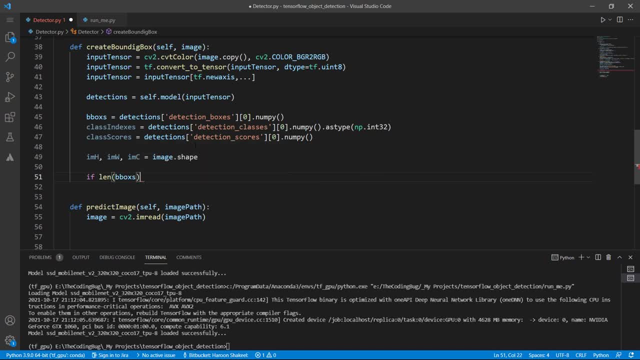 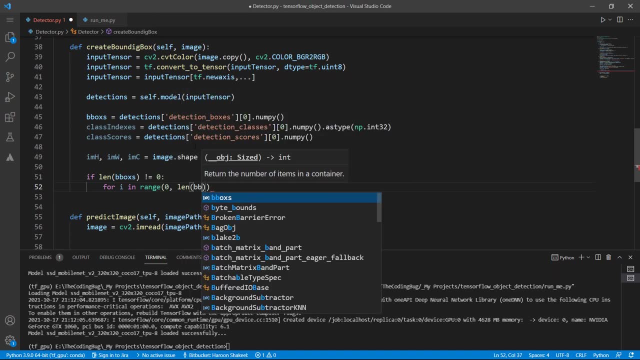 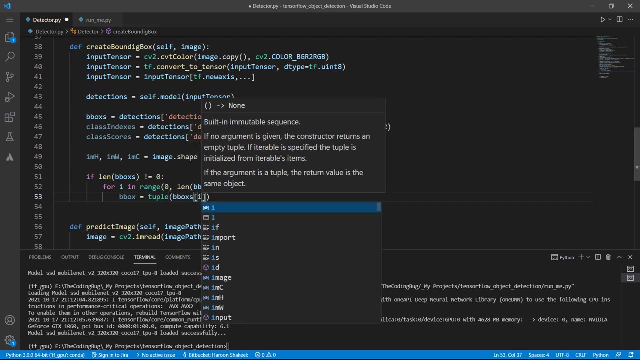 any bounding box in the image. we want to proceed with drawing each of the bounding boxes. we need a loop till the length of the bounding boxes array and at the index I we will be extracting one bounding boxes as a tuple for same index I. we also need to get class confidence. let's convert class. 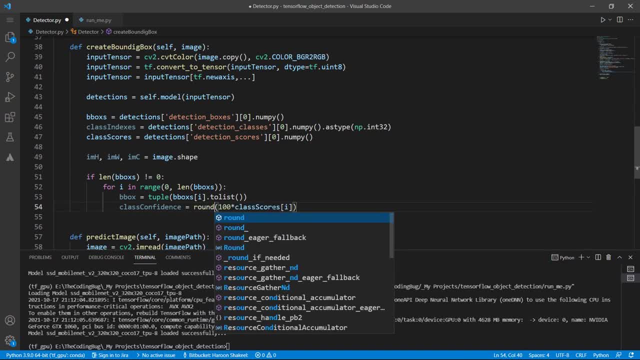 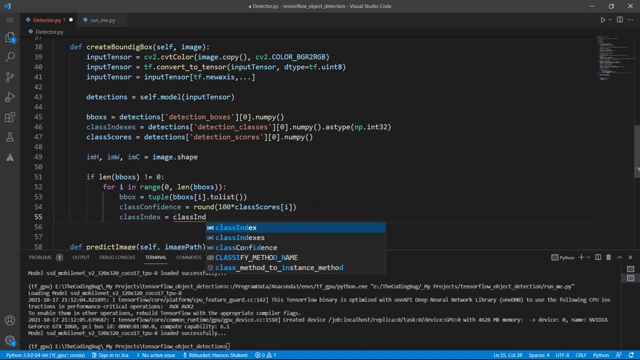 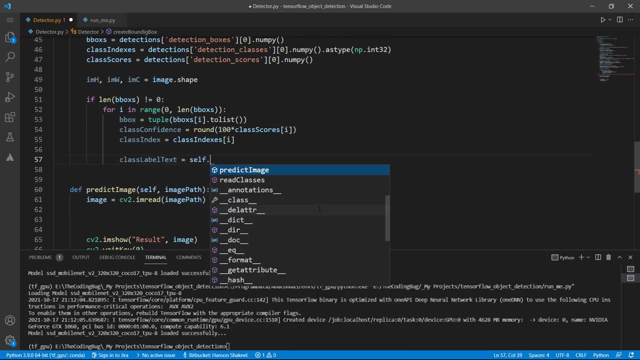 confidence to the scale of 100 and round it now against the class index. we need class label from our classes list and we also need to get the color that we defined against that particular class. so we need to do that. the last component: I need to close it, so I add the. 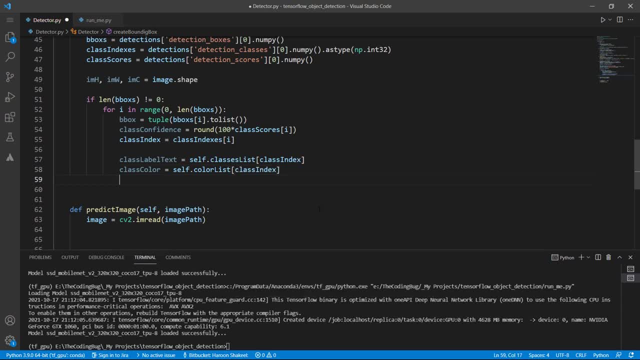 fifth component, which is to take ourуса1.x, the last chart from each of the boxes of our smaller Chinese, and then it will do, is a clean boundings, now bags, and now we need to get distribution research. so the first part was about location and 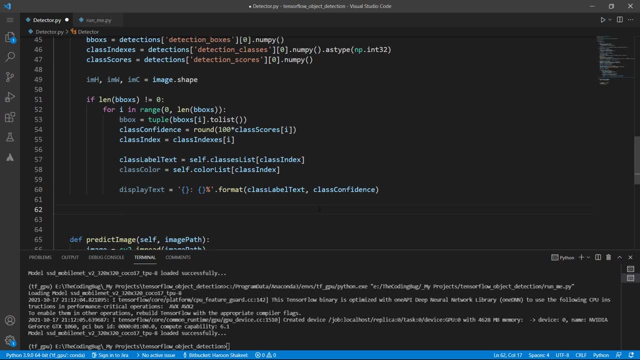 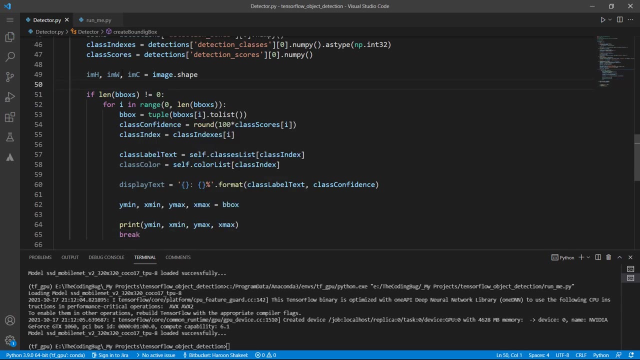 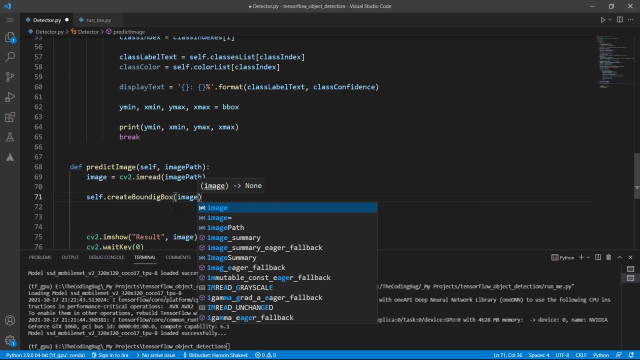 the standard and xmin by max and xmax values. let me print these values to show you what we have got here. let me put a break here to end the loop. after first iteration, let's call the create bounding box method here in predict image, and it will take image as a parameter. all right, let's run. 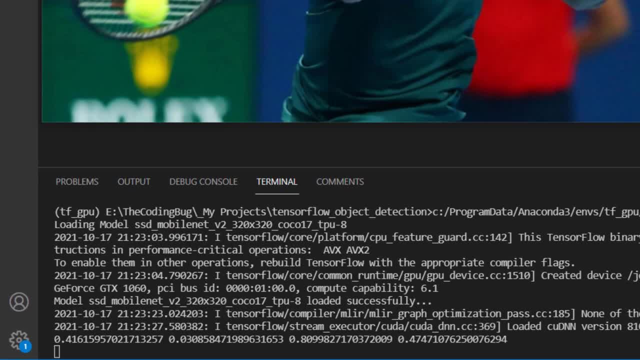 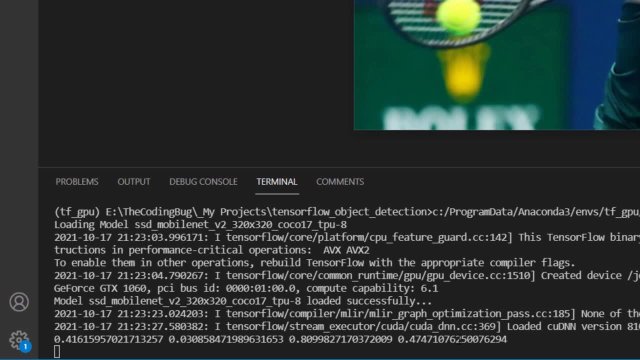 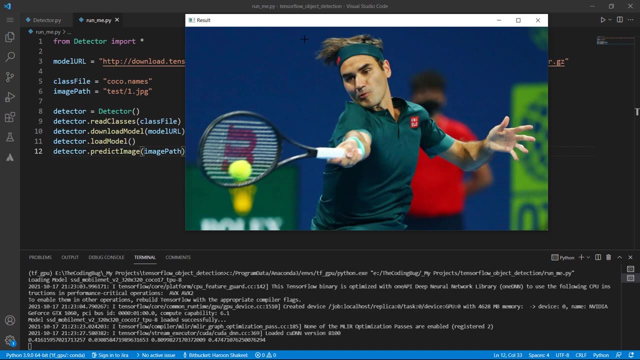 the main file and here you can see all four values. these are basically coordinates of the bounding box, but these are relative to the height and width of the image and are not absolute locations. so we can get actual pixel values or actual locations of the pixels by using the width. 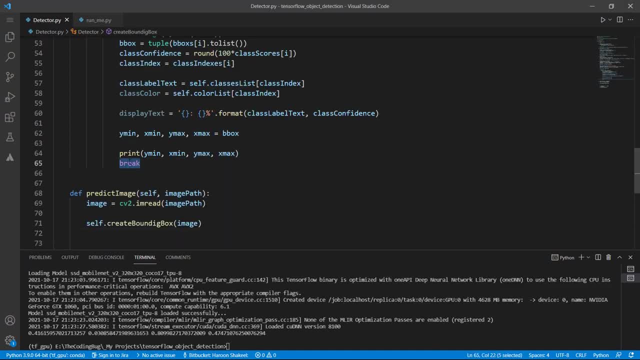 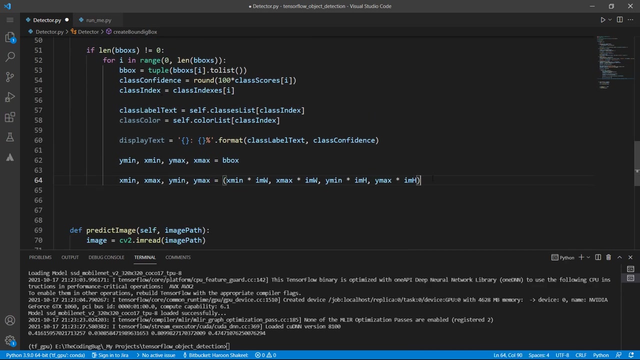 and the height of the image. let me show you how. so let's remove this break and print statement. we can get actual pixel locations of xmin by multiplying xmin with image width, xmax location by multiplying xmax with image width, ymin by multiplying with image height and ymax by multiplying with image height. also. 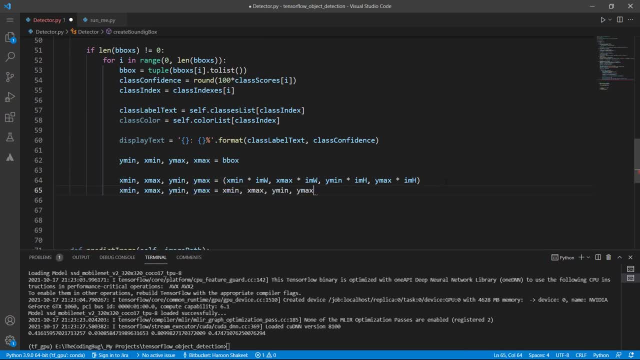 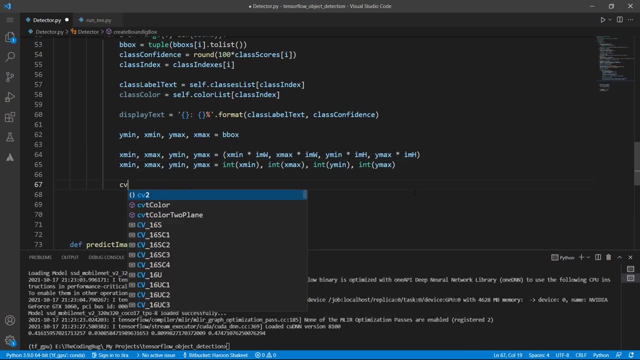 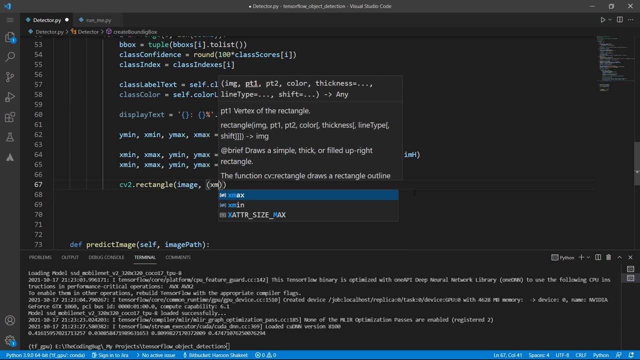 and of course it would give us a float value, so we need to convert it to integers. there you go. now let's call cv2.rectangle method and pass image to it. then starting point of the rectangle, which is xmin and ymin. then ending point, which is xmin and ymin, then ending point. 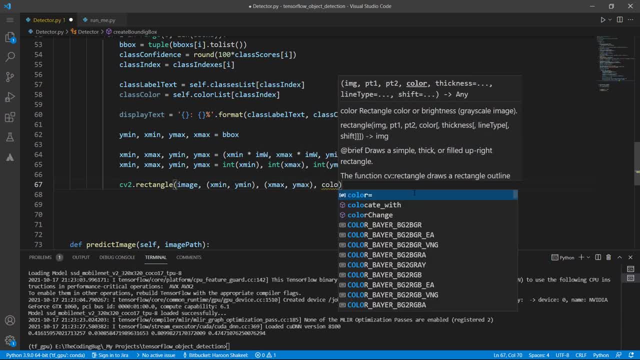 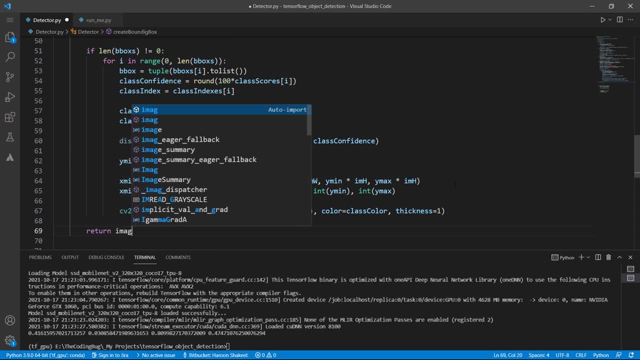 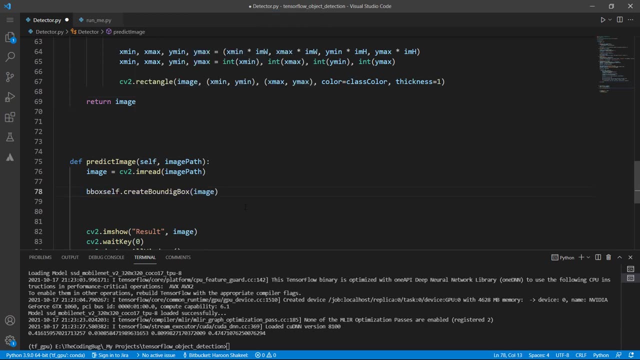 which is xmax and ymax. color of the rectangle would be class color that we have extracted above, and thickness would be one. let's return this image on which we have drawn all the bounding boxes. this function now returns the image, so let's call it bbox image and let's 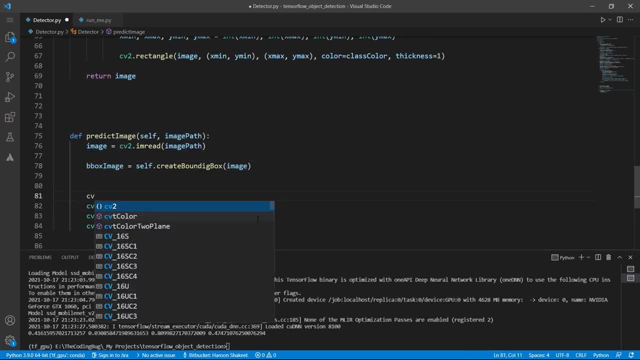 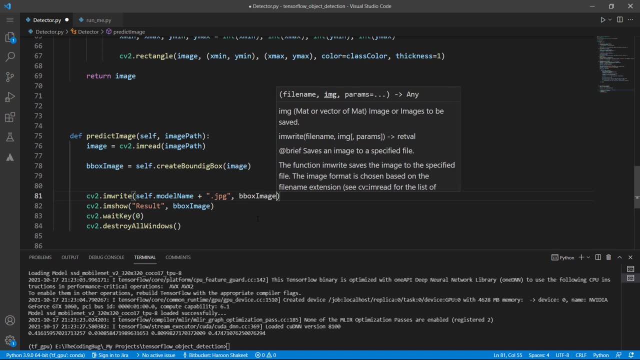 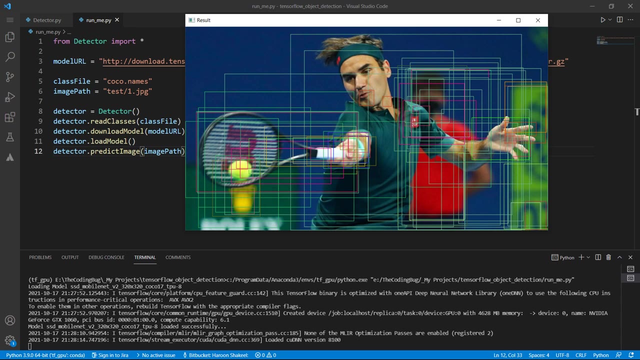 show this here instead of original image. we can also store this image with the name of our object detection model so that later we can compare the results. now let's run the main file and here we have bounding box for each class in distinct color. but there is a problem. there are a lot of overlapping bounding boxes. 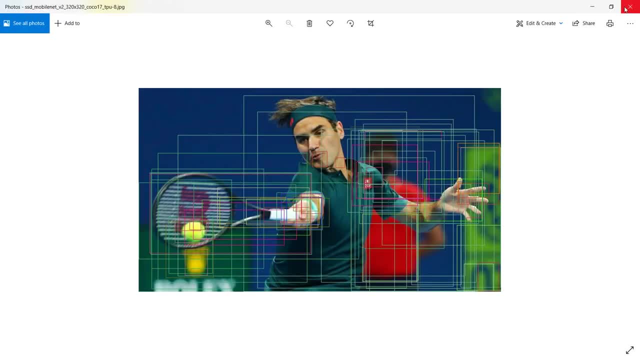 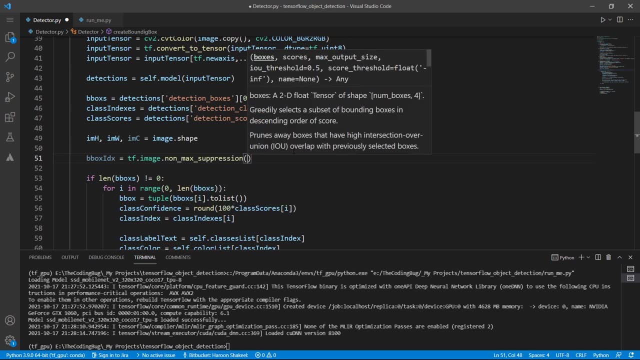 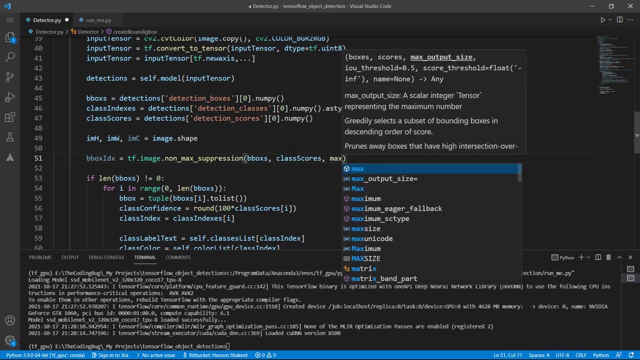 we can actually clean that mess by using non-maxima suppression. let's call tf dot, image dot, non underscore, max underscore suppression and pass the bounding boxes and class scores to it. then we need to define how many bounding boxes we want at max. so let's say 50 bounding boxes. 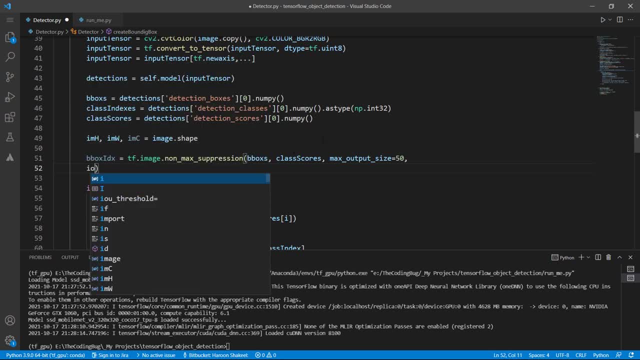 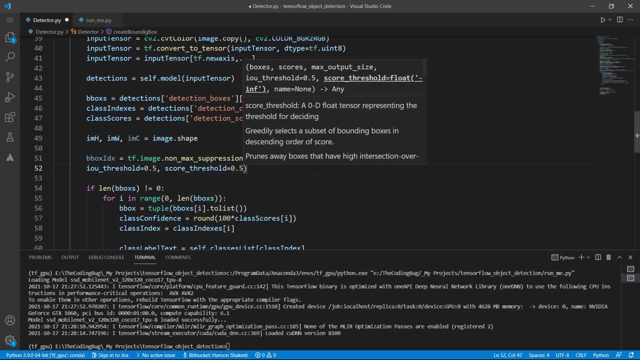 and then iou threshold, which defines the percentage of overlap of the bounding boxes that will be allowed. so make it 50. and then confidence score threshold of the bounding box. let's also make it 50 now. this would give us indexes of the bounding boxes that meet this criteria. 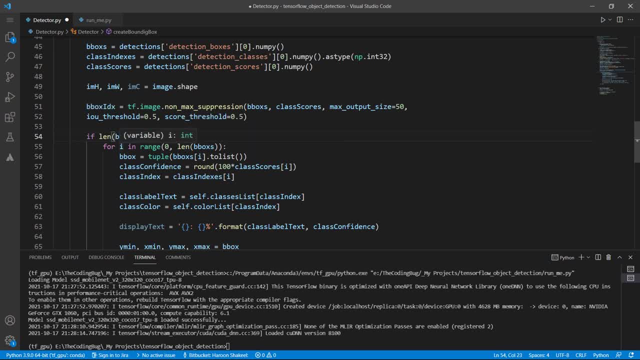 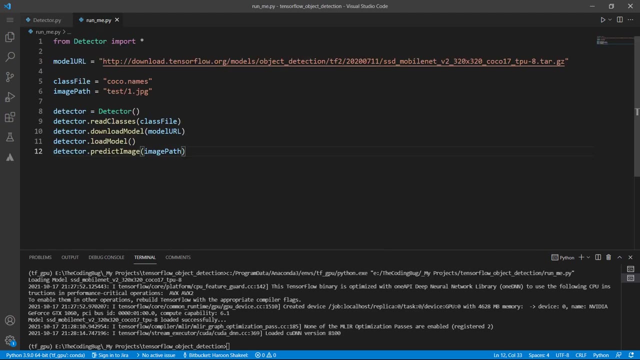 so now these checks would be based on this new bounding box index and in the for loop we want to draw the same bounding box returned by non-max suppression method. let's also print the bounding box indexes here. so here we can see now that only those bounding boxes are drawn, which. 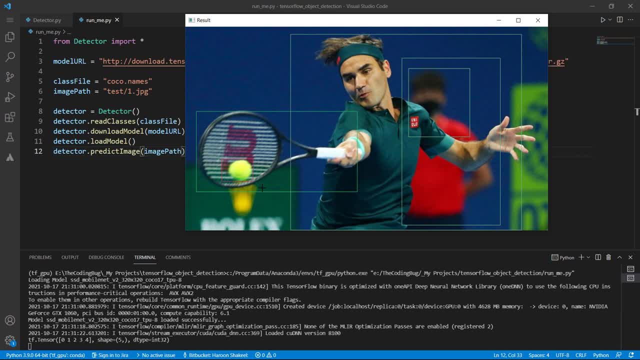 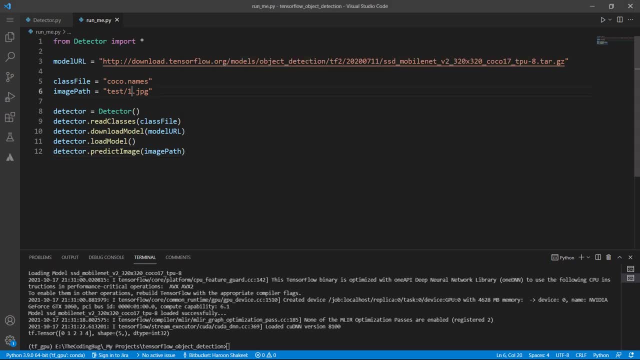 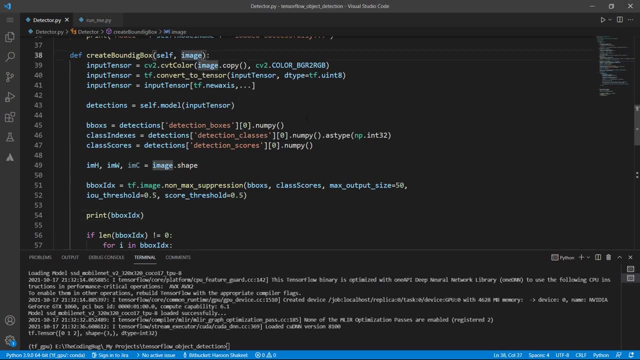 had a confidence score of 50 percent and an overlap of less than 50 percent, and those were the bounding boxes: 0, 1, 2, 3 and 4. let's change the image here, and here we have the result. let's make this threshold a parameter to be passed to our methods so that we can control it from the 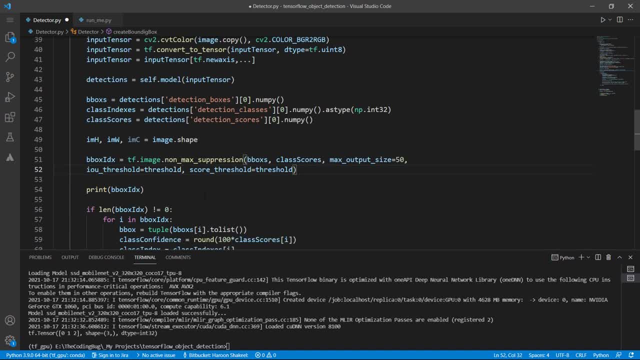 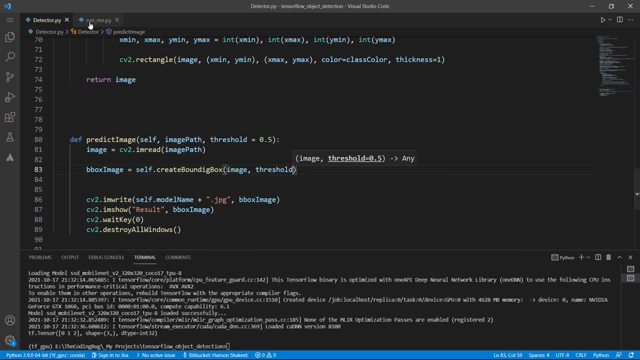 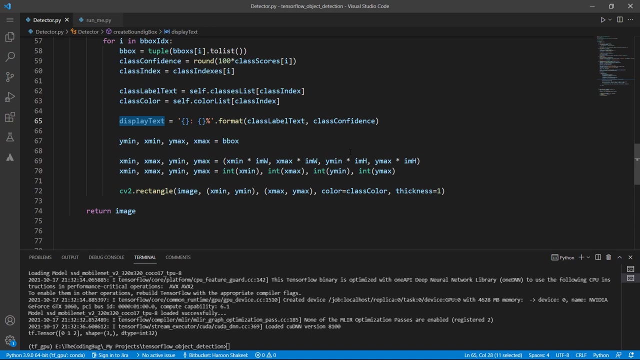 main file, these hard-coded values will be replaced and this predict image now takes the second parameter as well. let's create another variable here and pass it here. okay, it's just for the convenience for later use. all right, now we need to put the class legendary confidence text on the bounding box. 6, 18. 4, because text method pass image and location would be x. lemme go ahead and leave as theевой touching text or text method, but a little above y min. so minus 10 pixels above the founding box. but work, define font size. it's going. 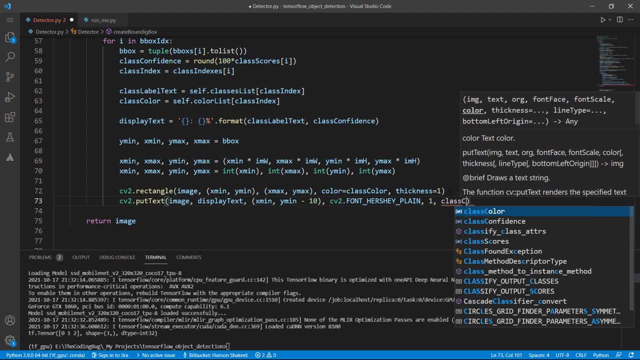 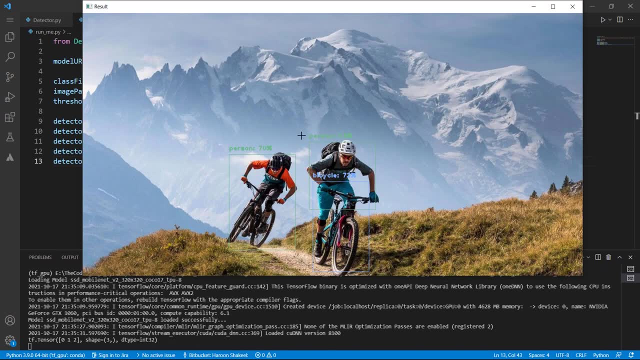 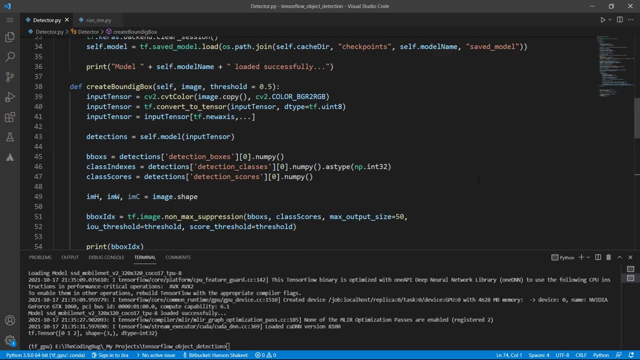 color would be the same as class color and thickness of 2. Here we have the label and confidence scores as well. But if you do not like the colors of the bounding boxes, We can change this numpy random seed to get different set of colors. I'm changing it to 20. 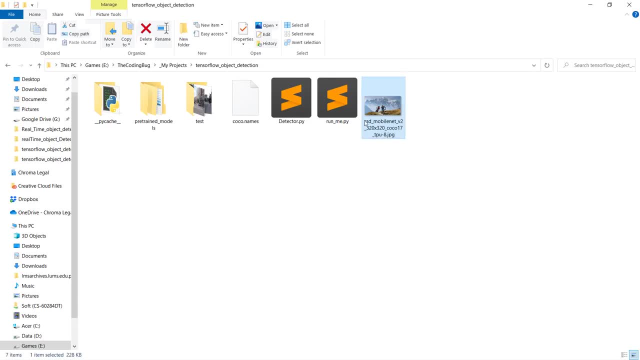 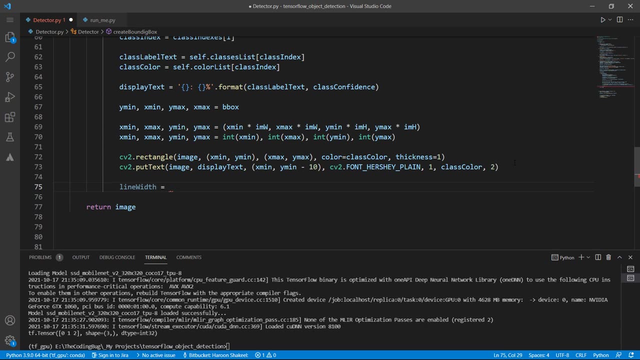 I also want to beautify the bounding boxes by making the corners a little bit bold. so we will draw a small line in the corners and the line width would be proportional to the size of bounding box in pixels and we can get the size of bounding boxes in. 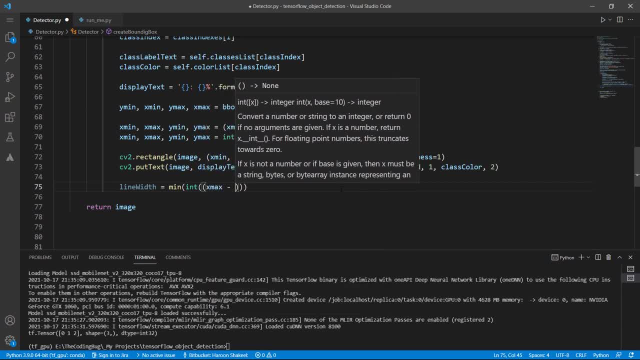 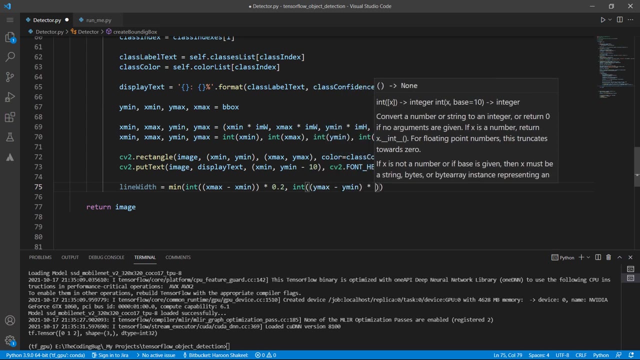 x-axis by subtracting X max and X min and then multiply it with 0.2 to get the 20% of this size and Of course then convert it to integer. same goes for the y-axis, and Once we have Both of these values, we want to get the minimum of these two. 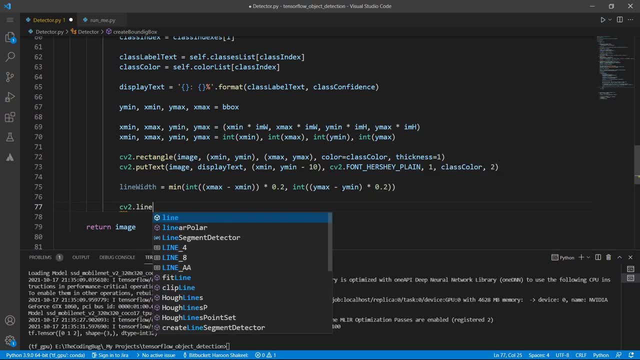 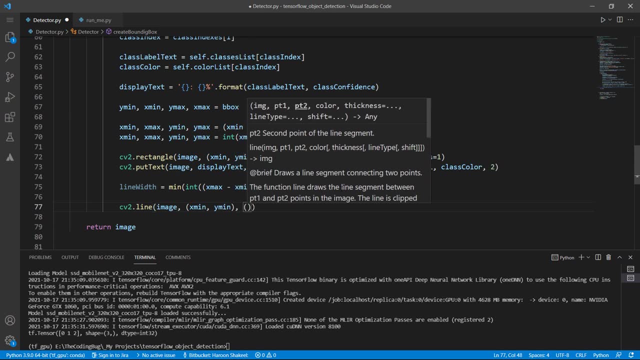 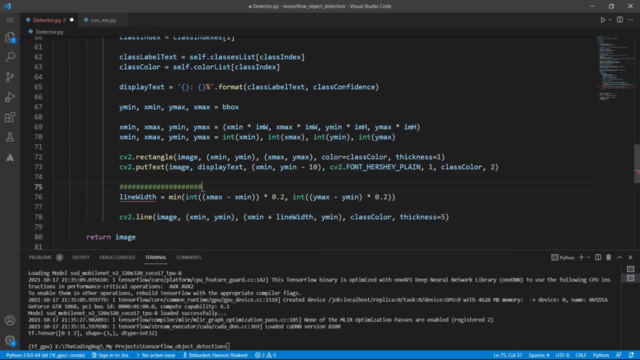 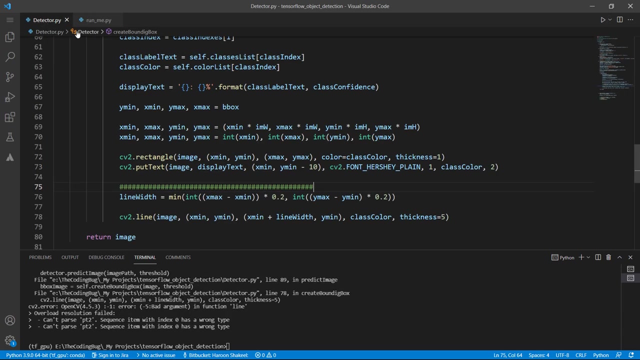 Let's now call cv2 dot line method. pass the image start position of the line, that would be X min, Y min and The end position, that would be X min plus line width and Y min. Let me put marker here: Run the main code. There is an error. we must have missed something. 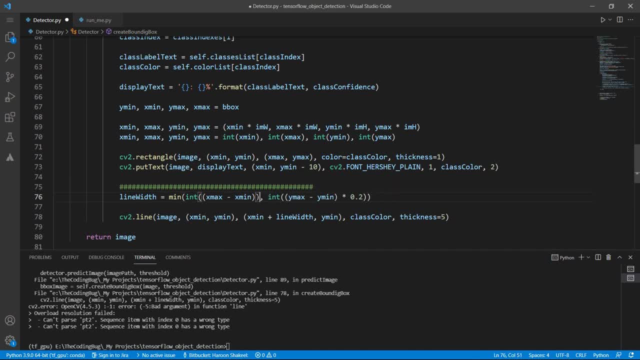 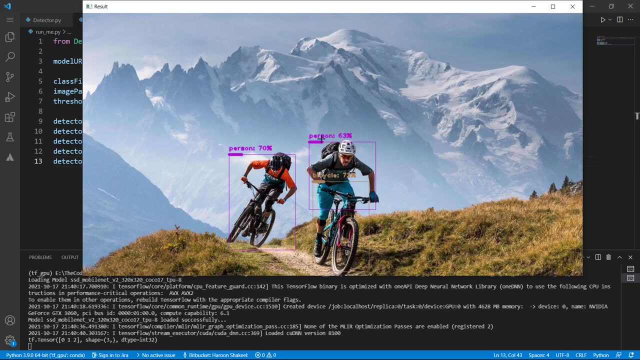 There it is. It's not integer. It should go inside the bracket here. There we go and We can see small line is drawn here. So this corner is basically X min, Y min. this one is X max- Y min and this one is X min- Y max. 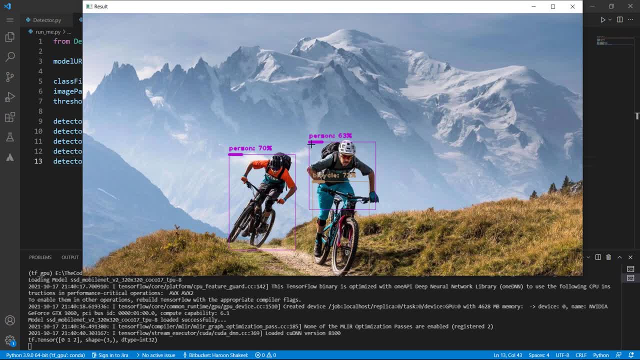 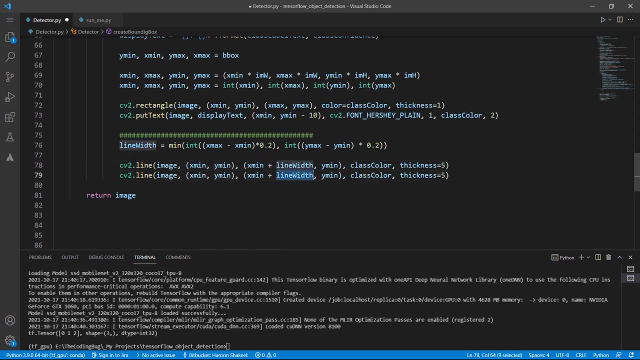 And final one is X max, Y max. so now, if I want to draw a vertical line here, I will have to draw from X min to Y min, plus line width width. let's copy this line and just change this to X min and this one to Y. 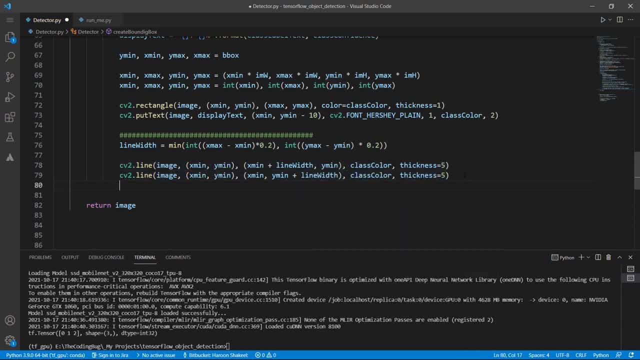 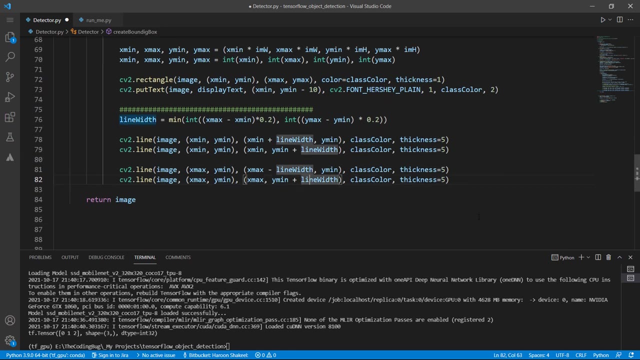 min plus line width. similarly, copy both of these lines for second corner. so X max- Y min, X max minus line width, Y min and X max- Y min, X max- Y- min plus line width. let's copy all four lines and paste here. I want to put marker here to 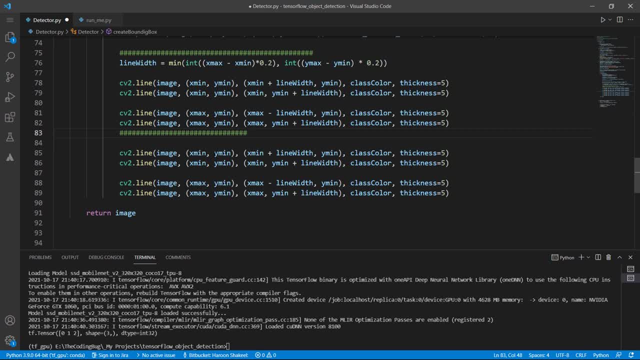 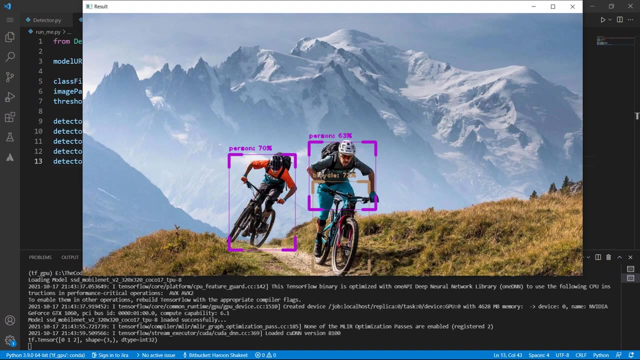 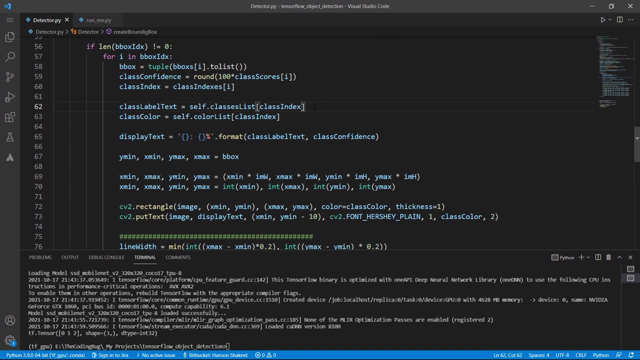 avoid mistakes, let me quickly draw other four lines as well. there we have it. let's run the code and we can see nice and pleasant bounding boxes. one more thing is that I want to this text to be in caps, so we can convert this class label text to: 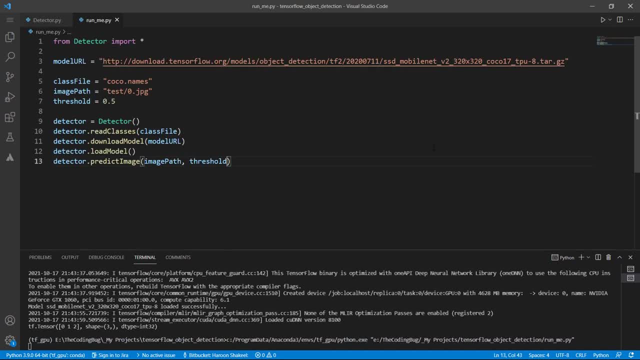 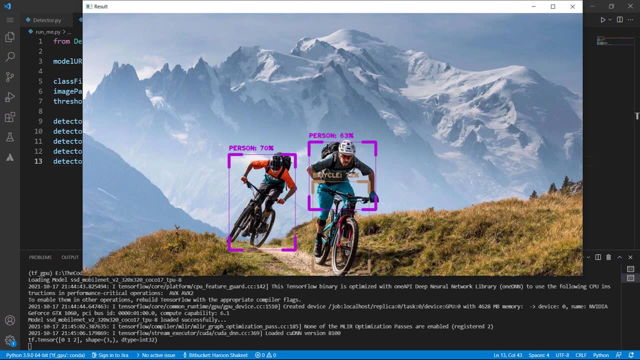 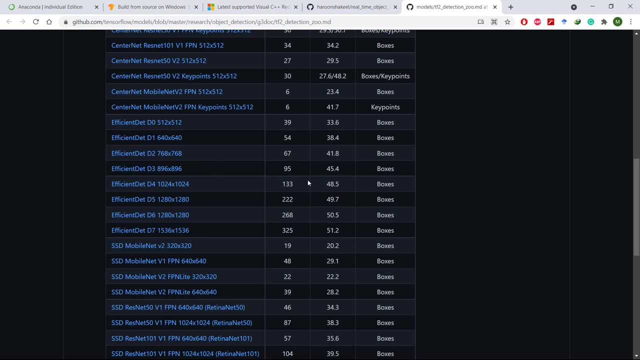 uppercase here now. if we run the code, we will see this great looking bounding boxes, but we can see that the backpack is not detected and this second bike is also not detected. so let's choose another model that is more accurate than SSD mobile net. let's pick this new state-of-the-art, efficient data. 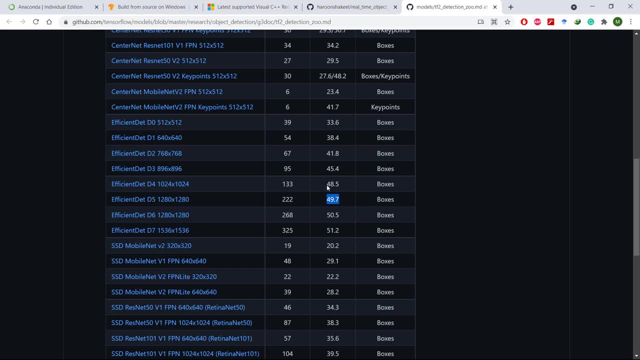 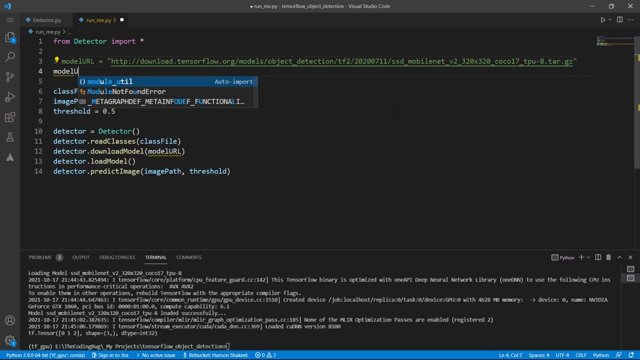 family. so d5 has just 1% improvement, but the inference time is double, so let's go with d4 instead. copy the link. let me comment this old URL so that we can go back to it later and replace model URL with this new link. let's run the code. 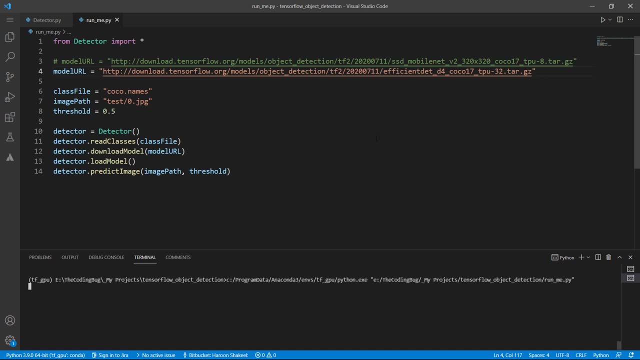 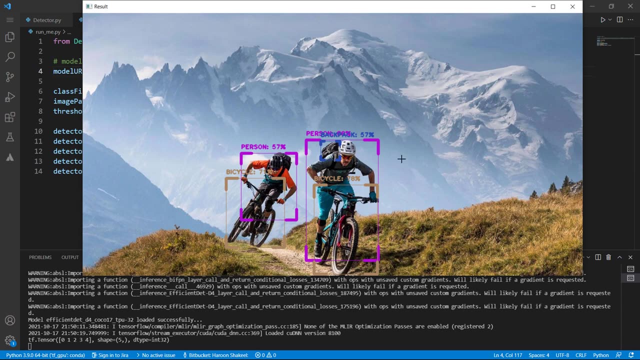 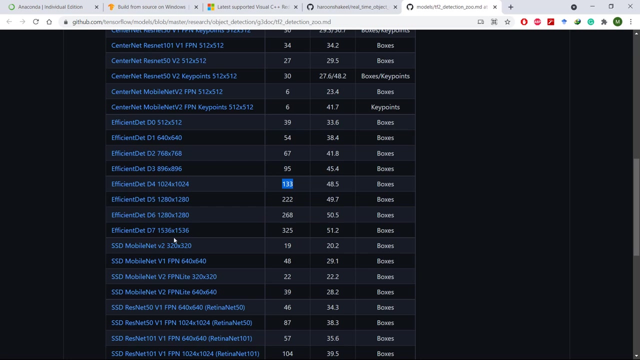 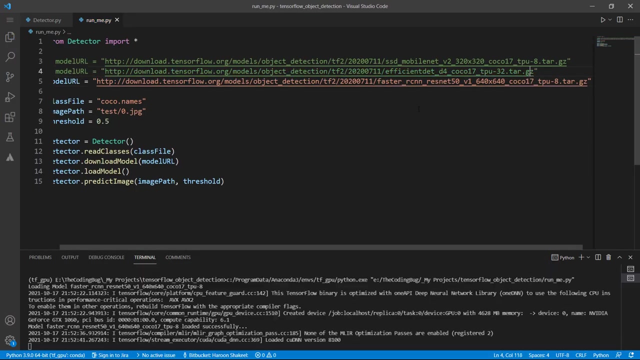 again. the model will be downloaded because it's not there in our cache. and here we have the results. now we can see that this backpack is picked up and the second bicycle is also picked up. let's quickly run another model. let's pick something from faster RCNN- this one- and paste the URL here. run the model and here we have object. 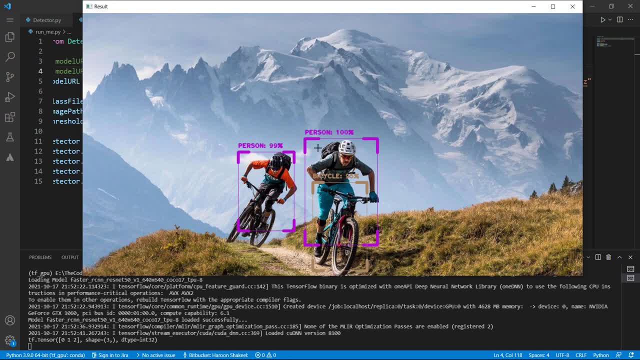 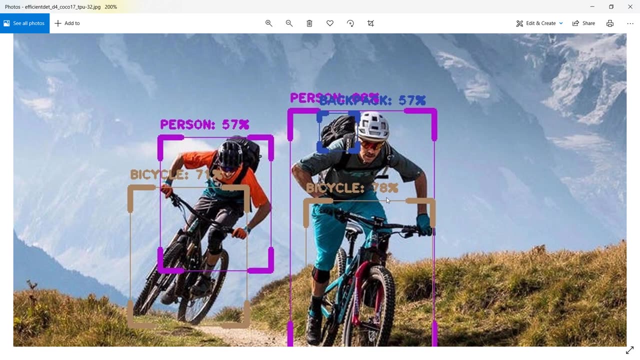 detection result for faster RCNN. this one does not pick up the bicycle, but its confidence is very high on all other classes that it has picked. so efficient debt picks up more objects accurately but has lower confidences. faster RCNN picks less objects but whatever it picked up has higher. 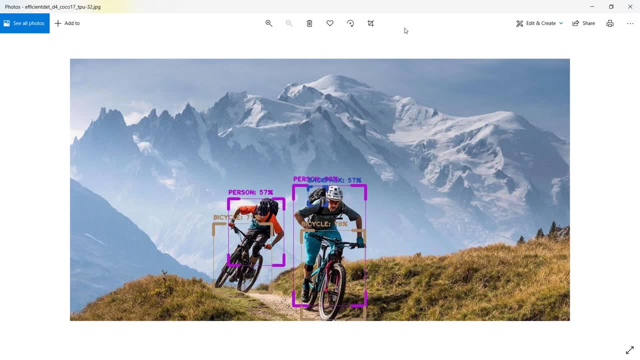 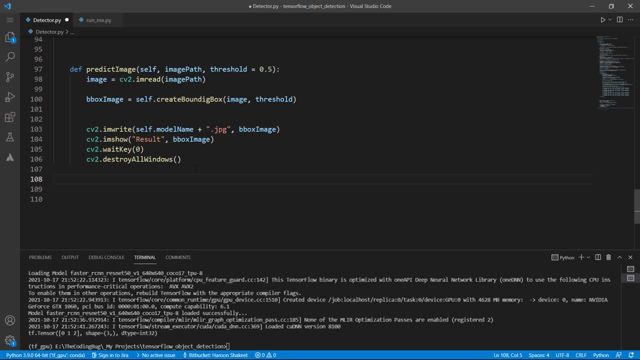 confidence almost 100%. SSD mobile net is somewhere in the middle. so interesting results all right. now let's run object detection on videos and webcams. for that let's quickly define a method called predict video, which takes video power as input, captured the video. if it cannot open the video, print error and return. 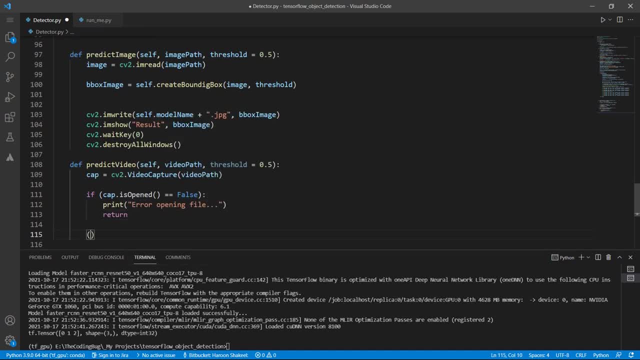 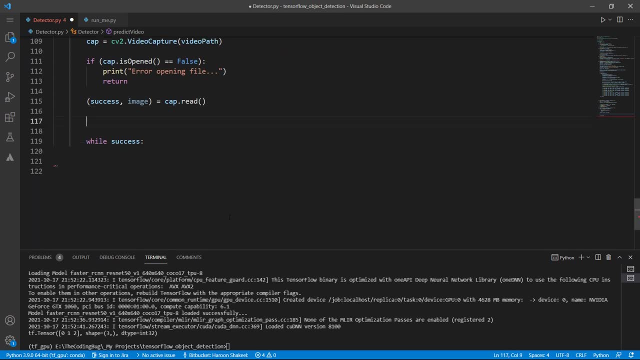 from the function. otherwise read the image, run a while loop if an image capture is a success. you know what? let's define FPS here also. so start time would be zero and current time can be taken from time module and FPS would be equal to the one over difference of current time and start time. start time would be: 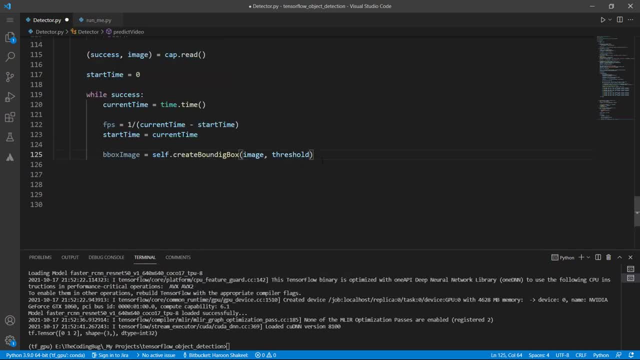 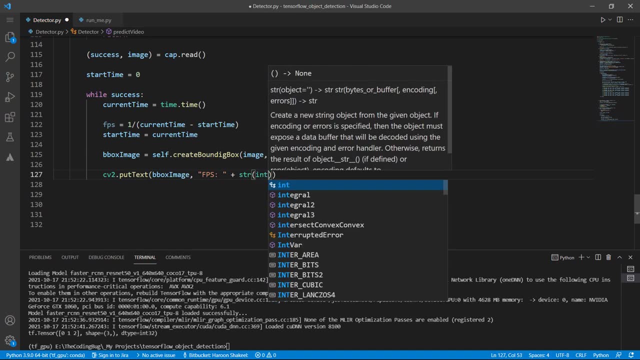 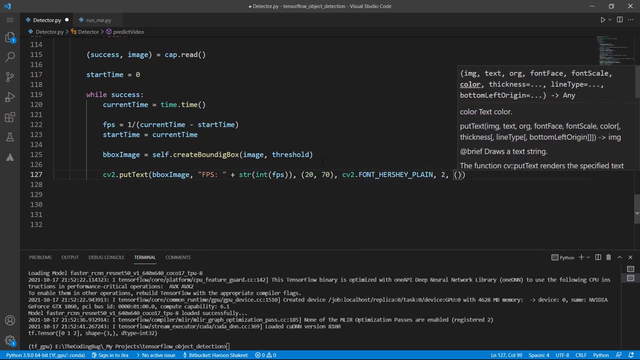 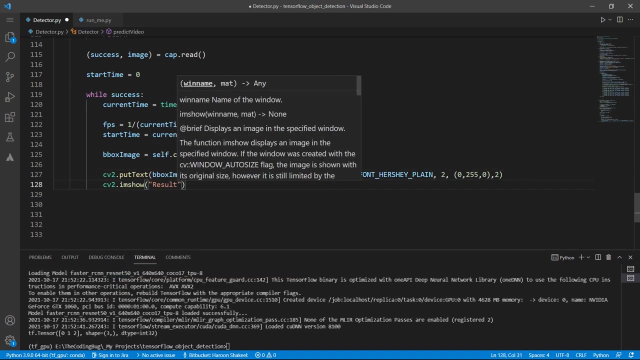 would be equal to the current time. Let's call create bounding box function on the captured frame, which will give us frame with bounding box, and we need to put the FPS on bounding box image in green color, which would be 0,, 2,, 5,, 5 and 0.. Let's show this video frame and we also need to.